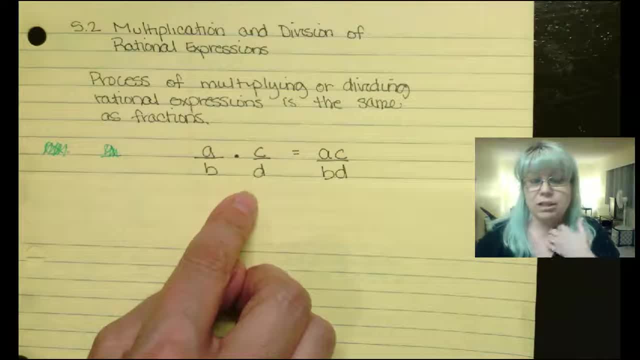 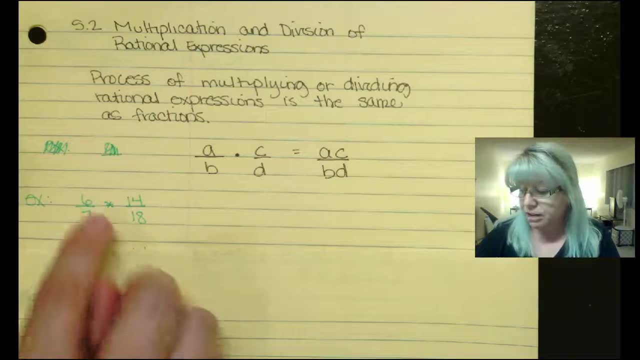 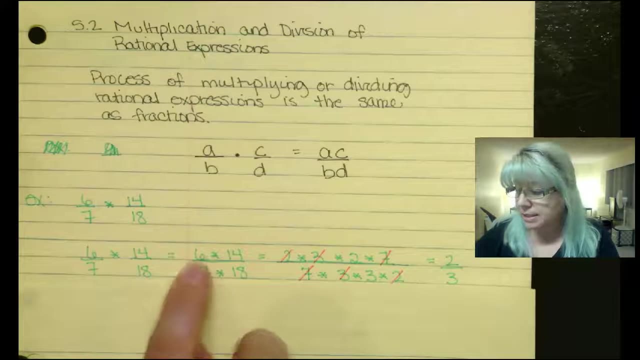 by the reciprocal for division. we're going to do the same thing for rational expressions. So let's recall the process for multiplying fractions. So let's say I have a fraction of 7.. 6, 7ths times 14, 18ths, That means it's going to be 6 times 14 over 7 times 18.. What I can? 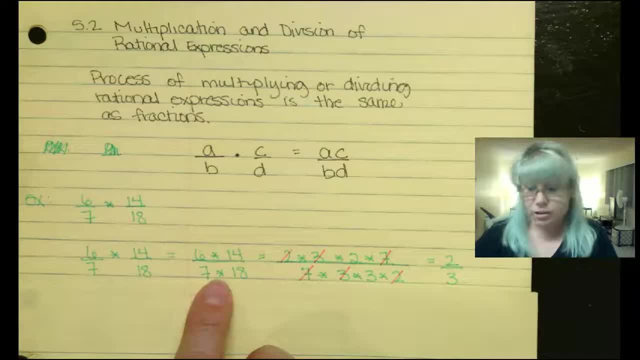 do is break down each of the values into its factors and then see what the numerator has as well as the denominator has. And I can reduce that because any value over itself, except 0 over 0, is a 1. So 6 can be broken down into. 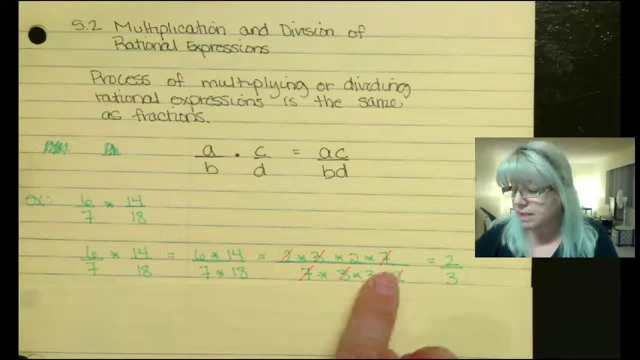 2 times 3.. 14 can be broken down into 2 times 7.. 7 is just a 7, because it's prime. 18 is a 3 times 2 times 3, or 3 times 3 times 2, or 2 times 3 times 3.. It doesn't matter what. 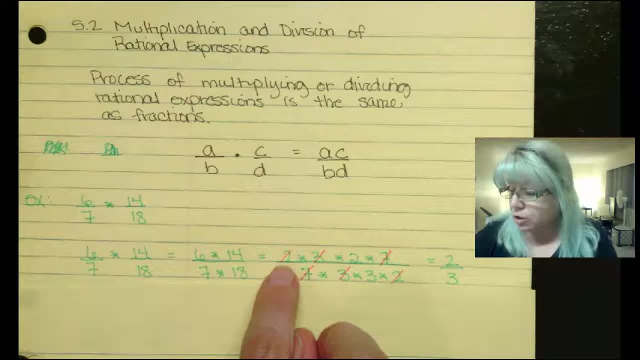 order. I can see in the numerator: I have a 2,, a 3,, a 2, and a 7, and the denominator: I have a 7,, a 3,, a 3, and a 2.. Because they share a 2,, a 3, and a 7,, that only leaves 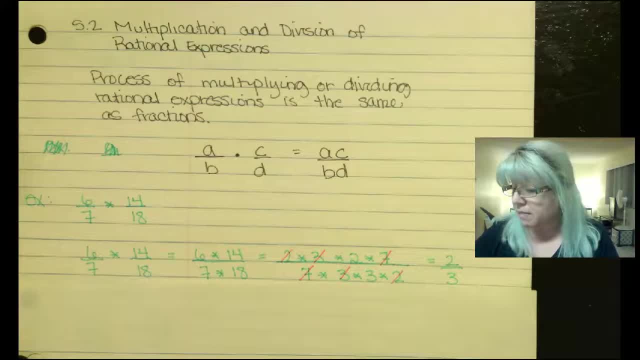 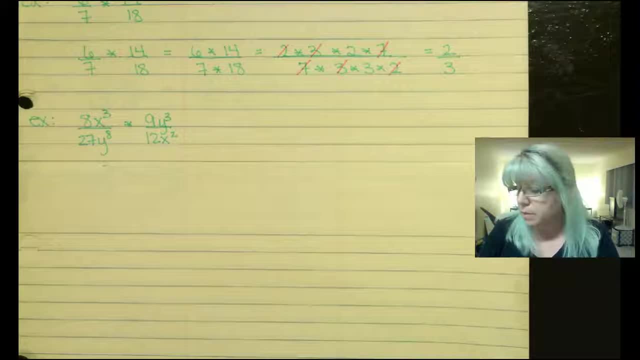 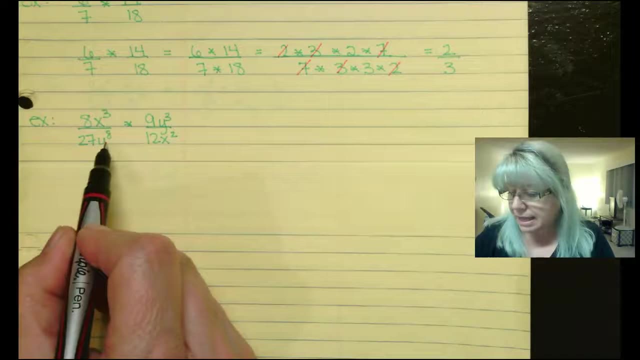 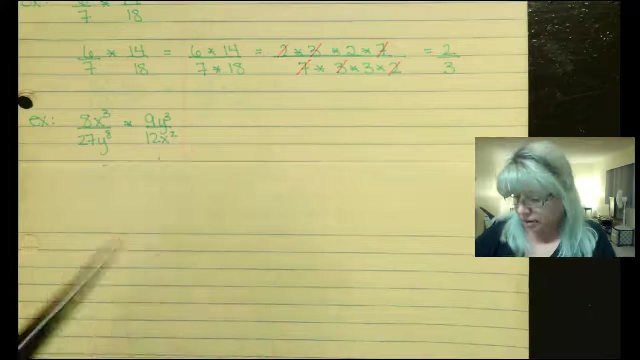 a 2 in the numerator. So my final result is 2 thirds. Alright, so let's try it with a little bit more complicated problem. I have 8x cubed all over, 27y to the 8th times 9y to the 3rd, over 12x squared. 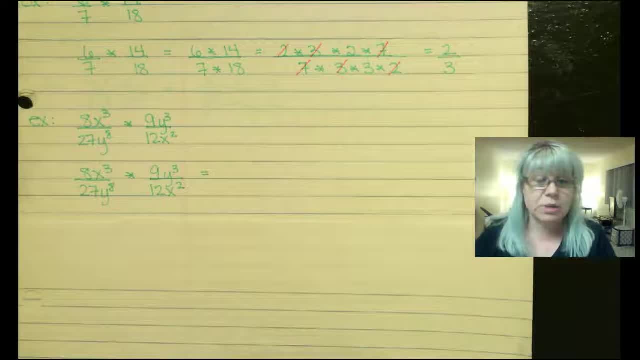 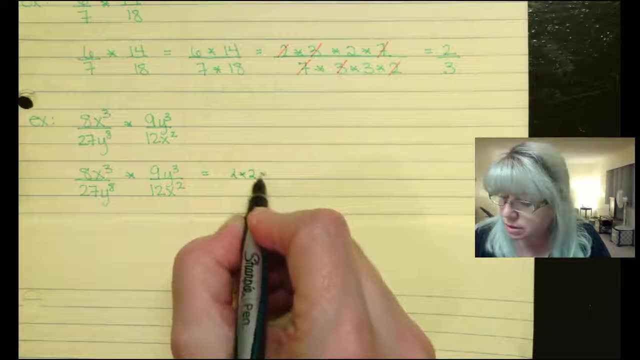 So the first thing I want to do is break these values into its factors. 8 is going to be 2 times 2 times 2.. x is just x cubed. I'm going to go ahead and leave it as x cubed. 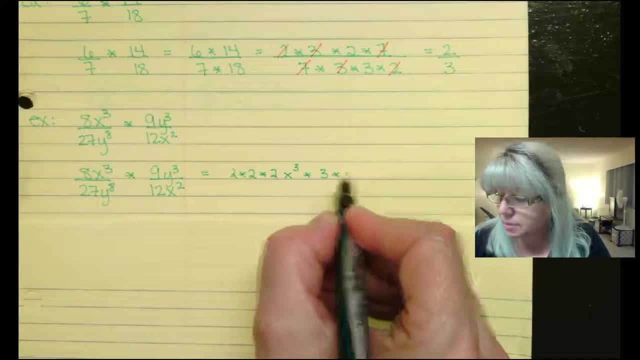 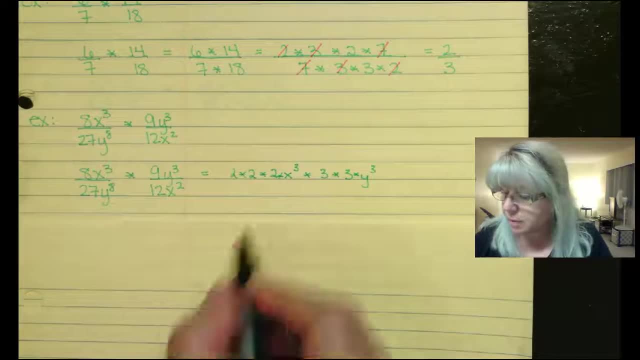 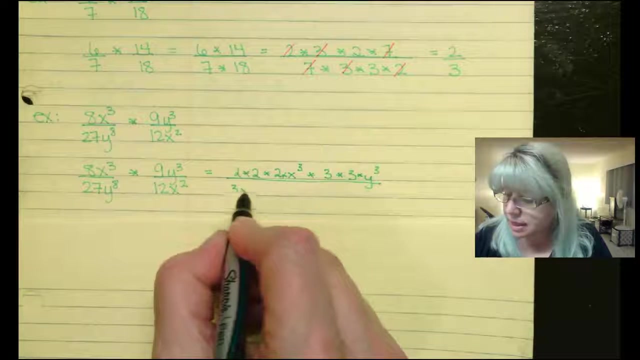 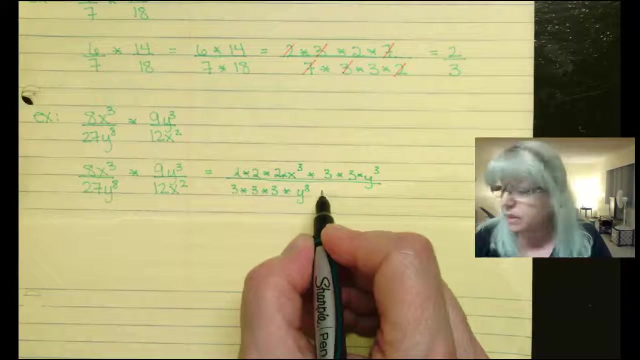 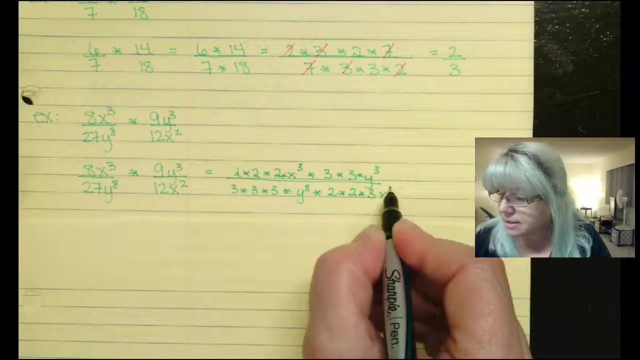 9 is 3 times 3, and y is y cubed. Be consistent there. That is all over. 27 is 3 times 3 times 3 times y. to the 8th, 12 is going to be 2 times 2 times 3 times x squared. I want. 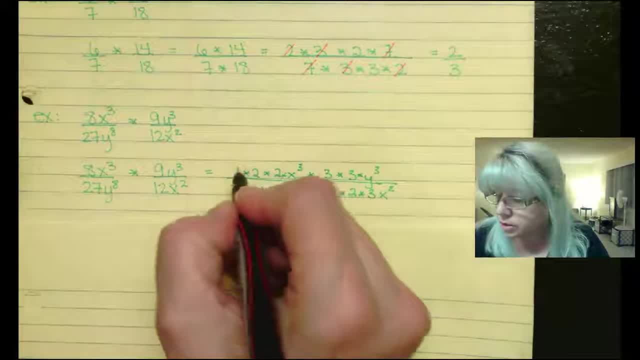 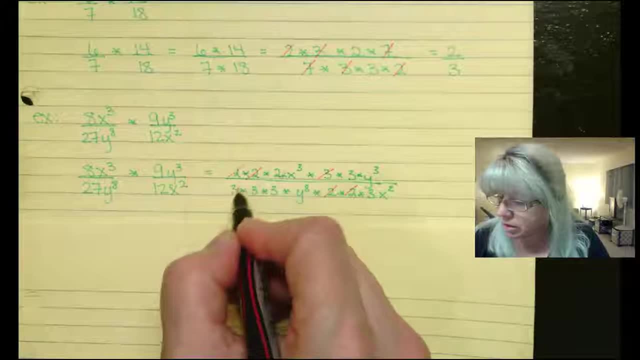 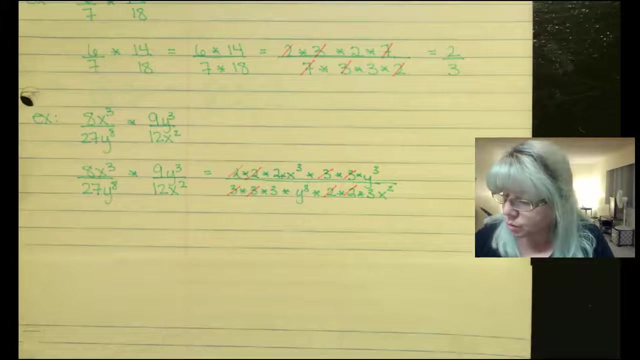 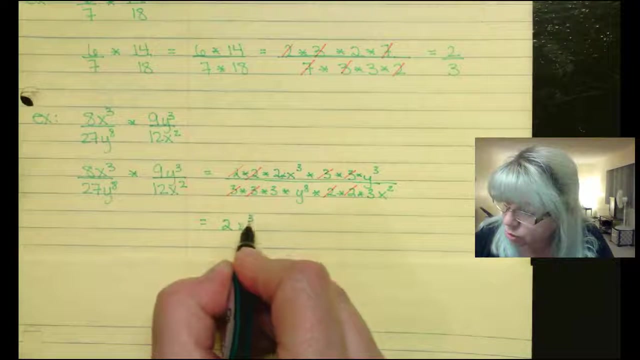 to reduce this as much as possible. 2,, 2,. okay, I have a 3 in the numerator, another 3 in the numerator, Okay. so let me just rewrite to see what else, so what we have left here. I have 2 in the numerator with an x cubed, y cubed. I have a 3 times a 3, which is a 9.. 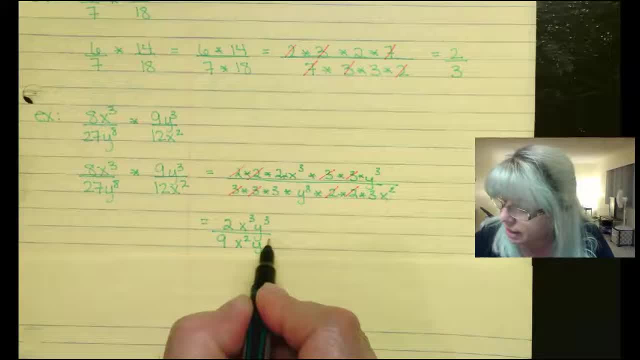 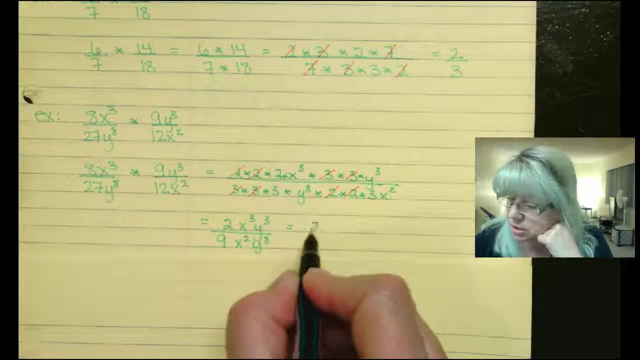 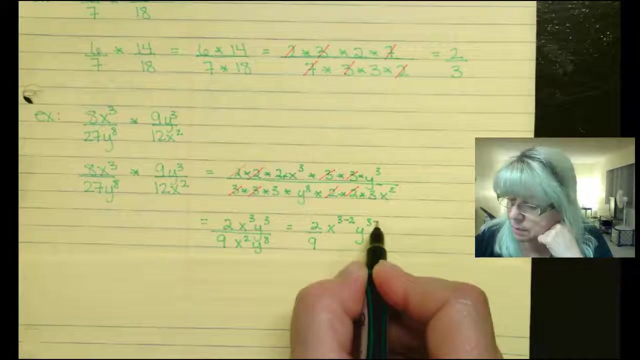 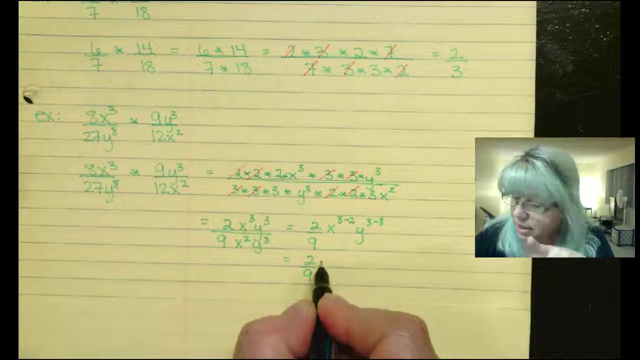 Let's see. I've got an x squared and a y to the 8th. Now I do need to remember my exponential rules here. That's going to be 2- 9ths, x, 3 minus 2, y, 3 minus 8, giving me 2 9ths, 3 minus 2 is a 1, y 3 minus 8 is a. 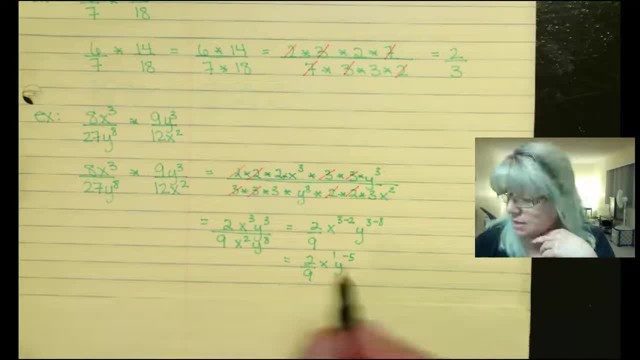 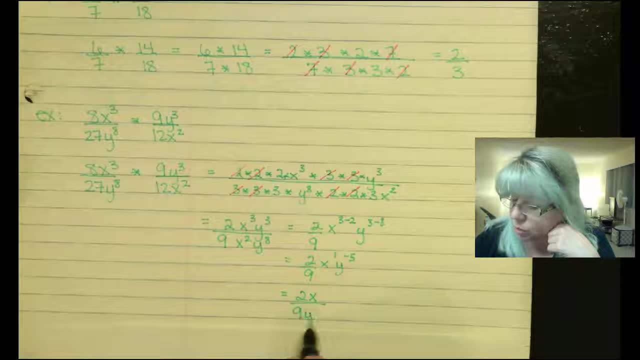 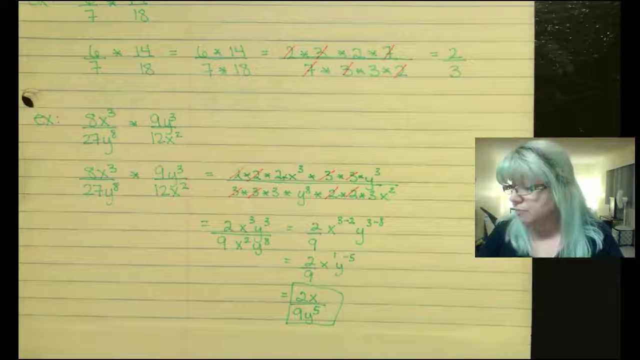 negative 5, but I don't want to leave my exponents in negatives, So let's bring the y back down to the denominator 6, all over 9y to the 5th. That is my final answer, My final. well, I suppose I did the. 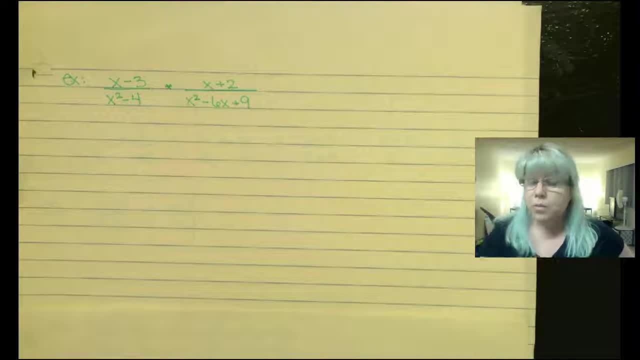 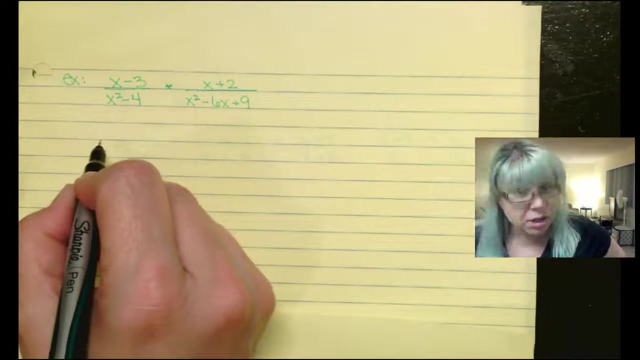 operation of multiplication as well as simplify. All right, for rational expressions it's going to be very similar. I want to figure out the factors and then see what the numerator has and what the denominator has. So let's factor each of the fractions, and I'm going to do that. 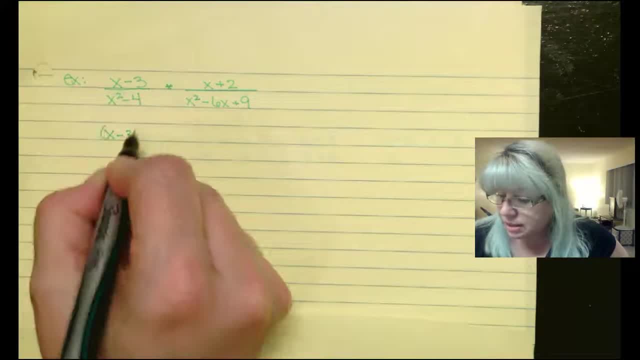 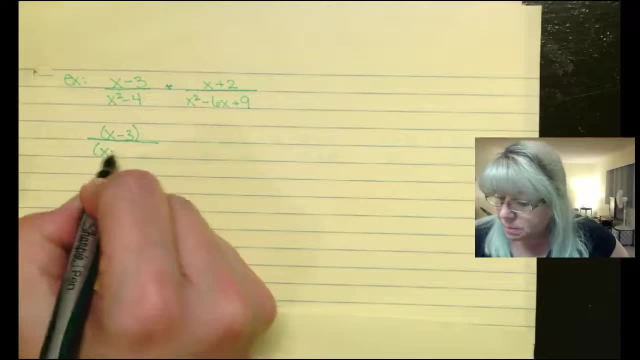 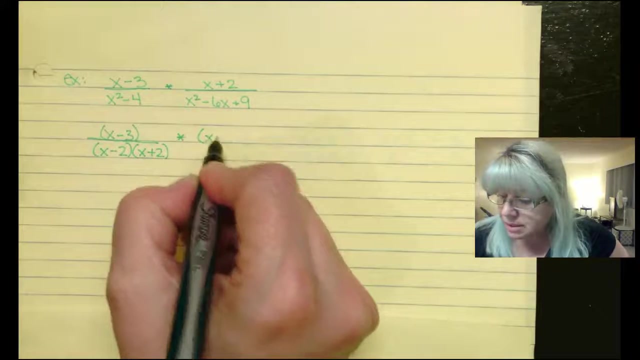 separately. So x minus 3, that's all I can do. Parentheses are just there for emphasis. x squared minus 4 is going to be x minus 2, x plus 2.. That is all multiplied by x plus 2.. Again, parentheses there. 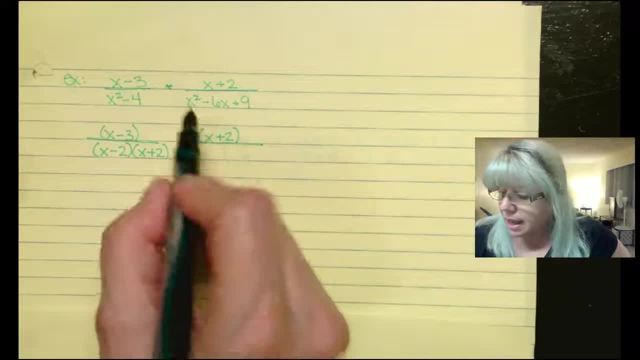 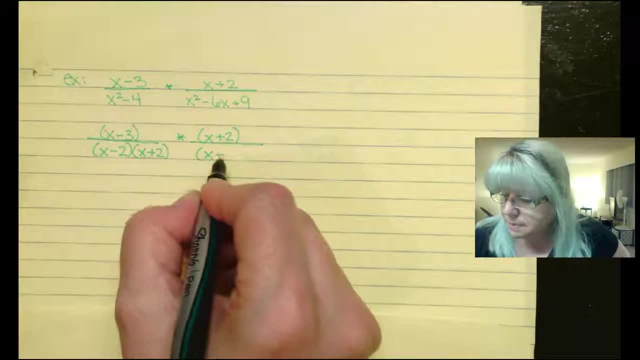 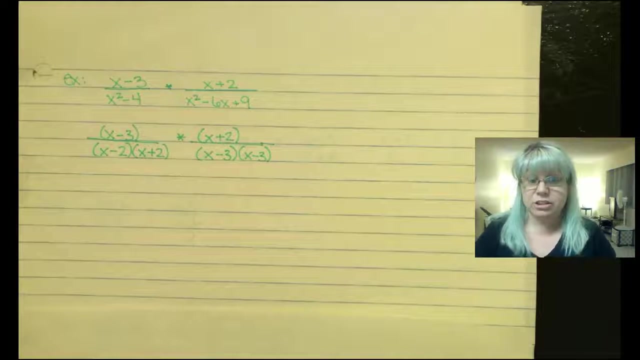 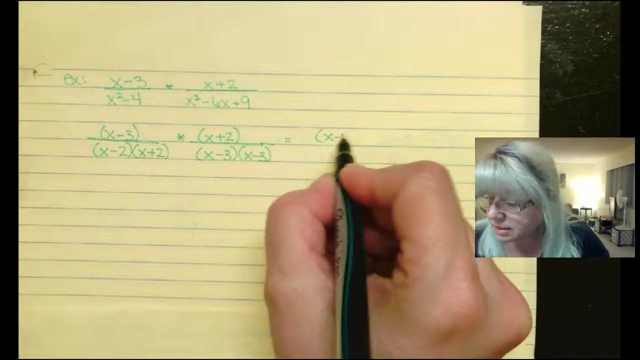 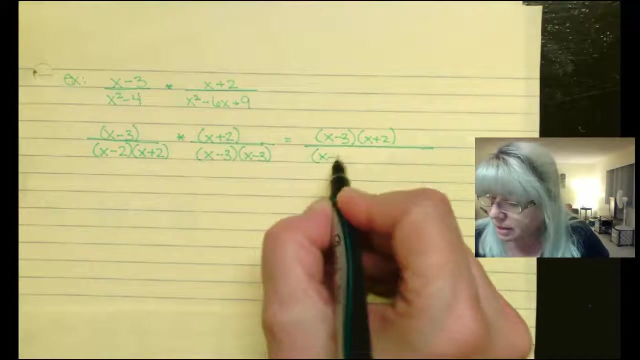 are, for emphasis, x squared minus 6x plus 9.. That is going to be x minus 3.. Times: x minus 3.. Now that I have it all factored, let's kind of squish it all in together, because it's all multiplication. Put it under one fraction: x minus 3, x plus 2.. All over: x minus 2, x plus 2.. 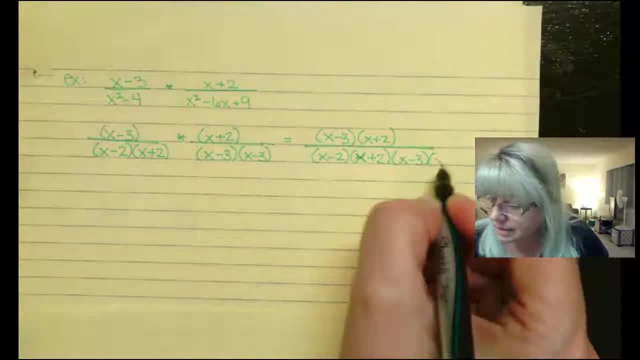 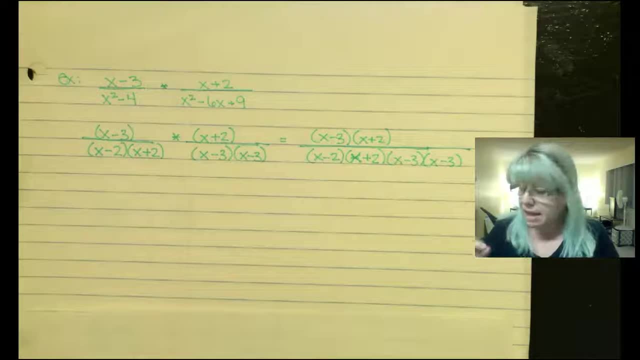 x minus 3, x minus 3.. As long as the numerator has the same thing as the denominator, it's a big fat 1.. So the whole entire x minus 3 over x minus 3 is 1.. x plus 2 over x plus 2 is 1.. The only thing left on top is a 1.. Therefore, 1 over x plus 2 is 1.. 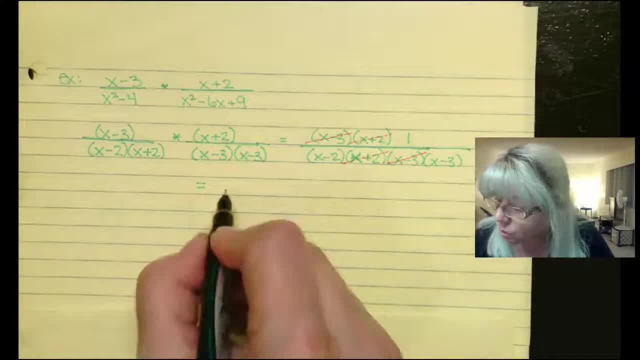 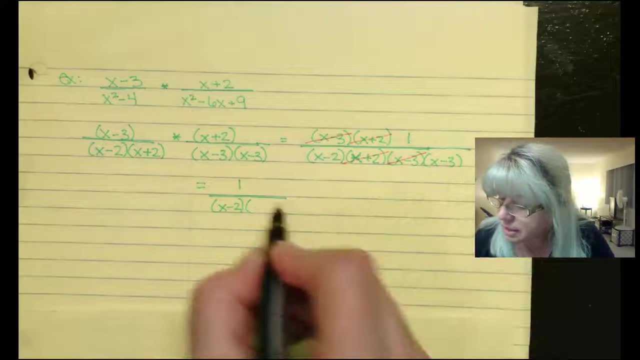 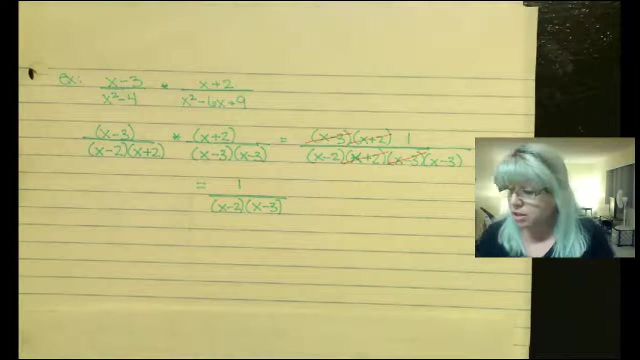 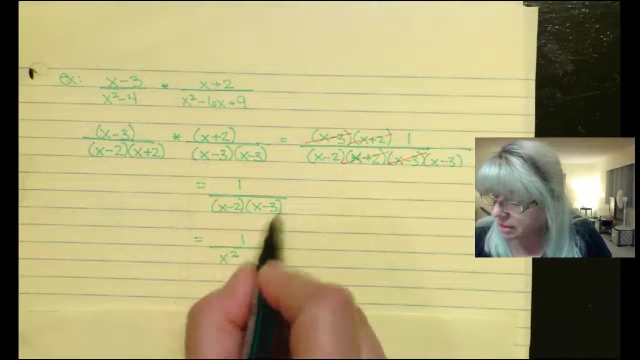 therefore 1 over X minus 2, X minus 3. that would be our solution. if you wanted to, you could multiply out the denominator. it's going to be 1 over x, squared minus 3, and a minus 2 is a minus 5x, and 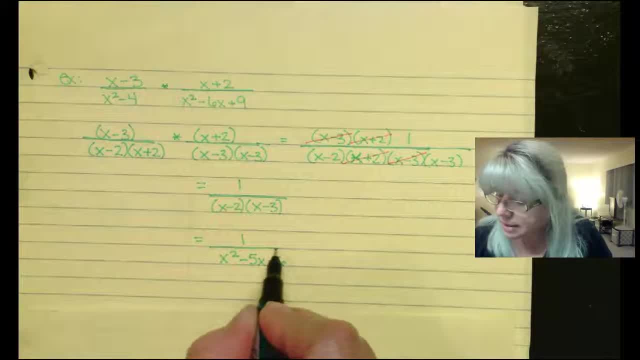 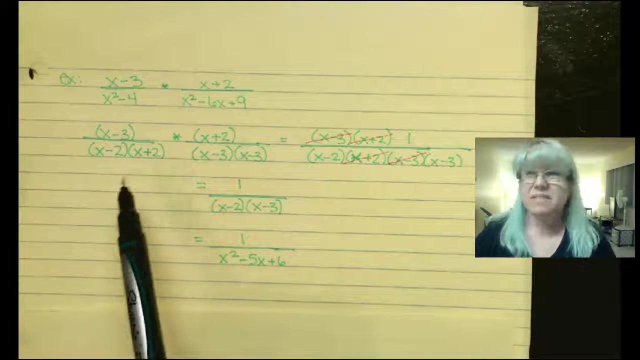 a negative 2. negative 3 is a plus 6. you don't have to do that last step. but yeah, that's the answer, right, not so bad. figure out its factors. reduce before doing the multiplication. it would be kind of difficult to figure out how we'd reduce if we did all the multiplication first. 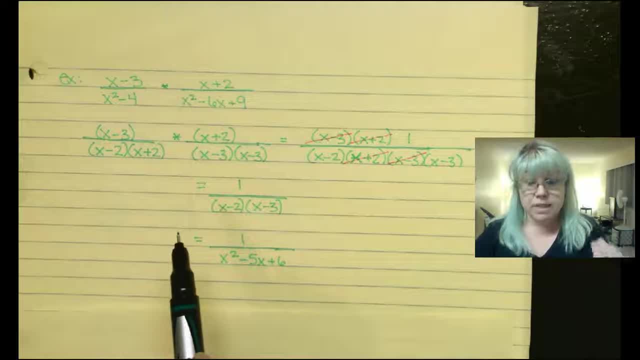 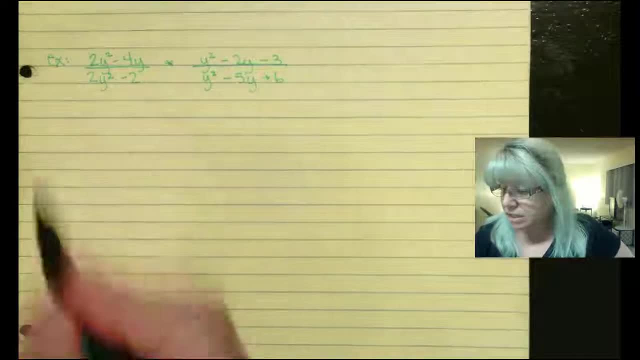 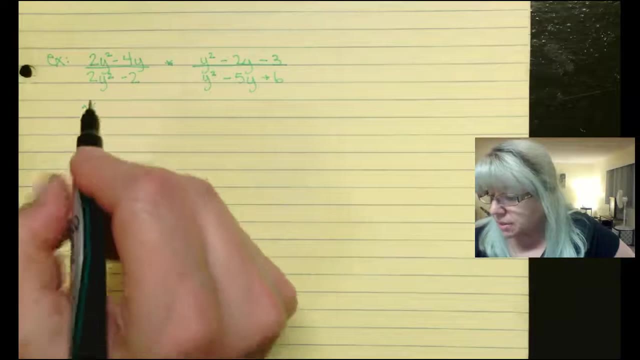 so figure out its factors, reduce and then do the final multiplication if needed. all right, thank you. factor first, I'm going to factor each of these fractions. all right, you might have to do it in a couple of steps. two: I can pull out. I can actually pull out a. 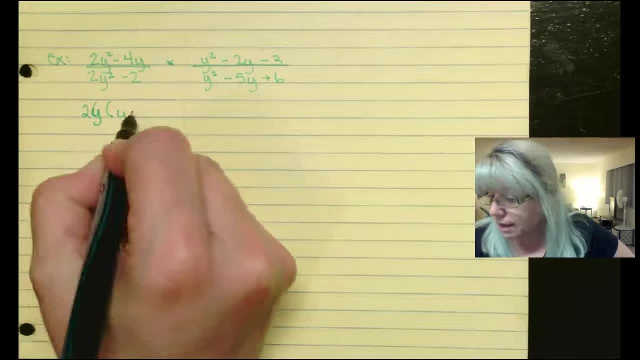 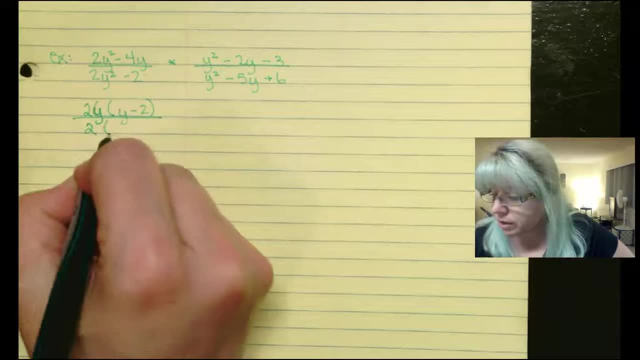 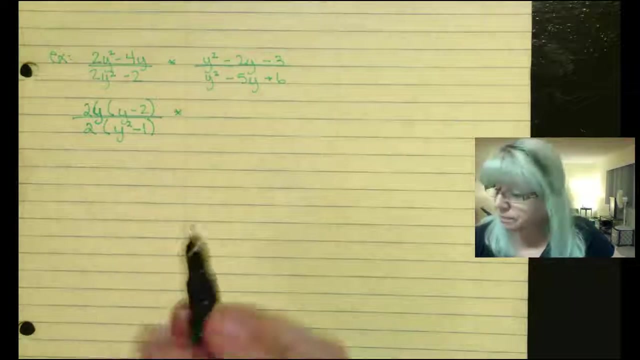 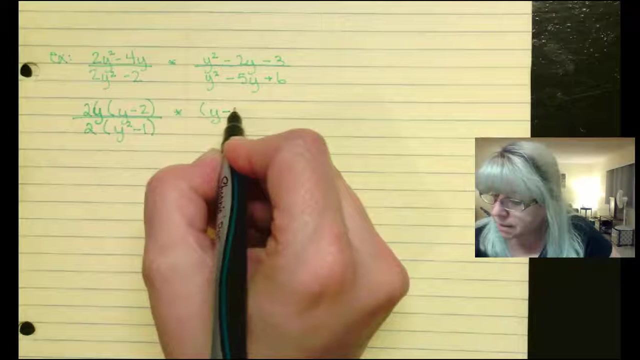 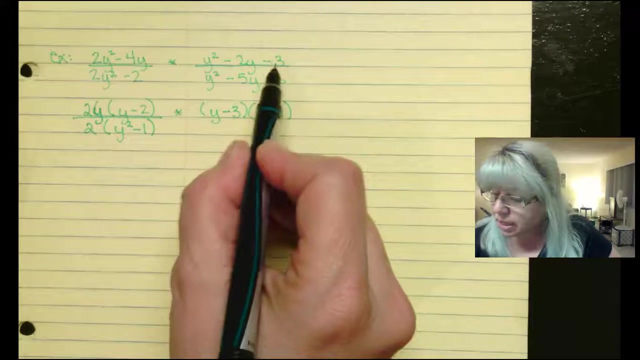 two Y leaves me Y minus two all over, and pull out a two here, leaving Y squared minus one. that's the first step for that one. let's see: Y minus three, Y plus one. negative three times one will give me negative three, and negative three plus one will give me the negative two right. 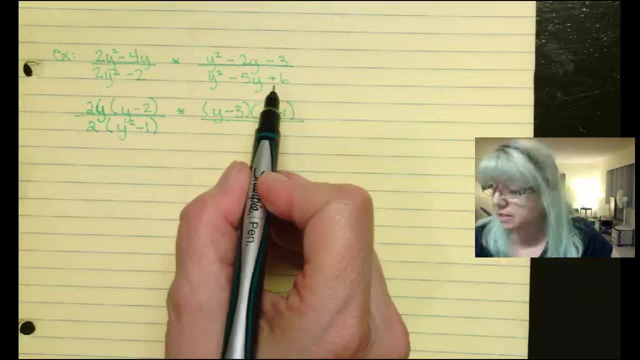 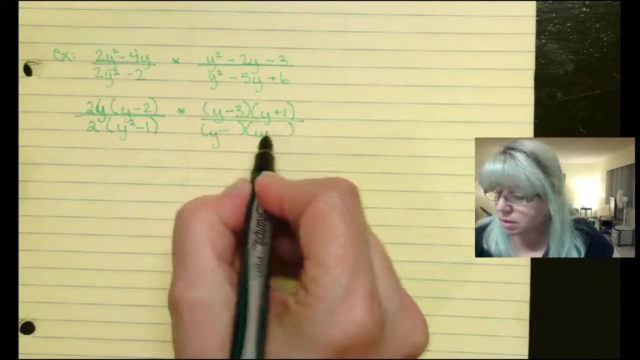 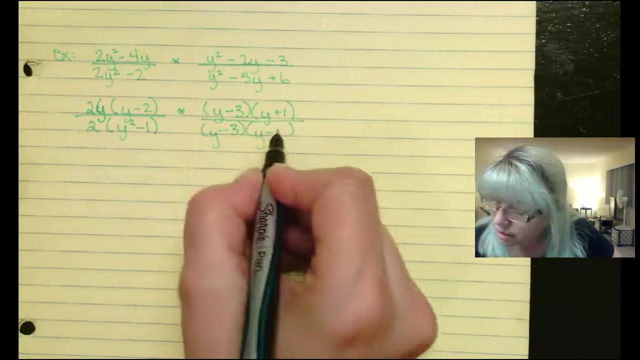 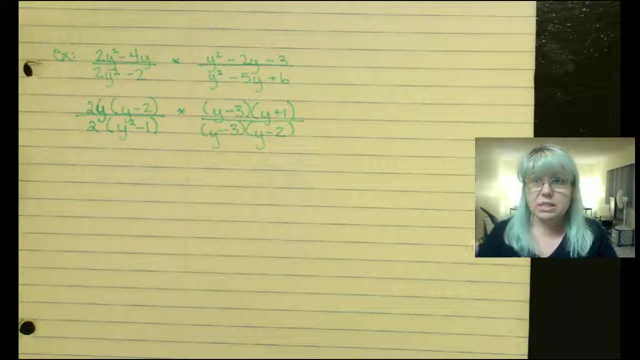 got a positive but a negative. therefore they're both negative. And well, 6 and 1 doesn't give me the 5, but 2 and 3 does give me the 5, and 2, okay. So I think the first thing I want to do is reduce the individual fractions first, and 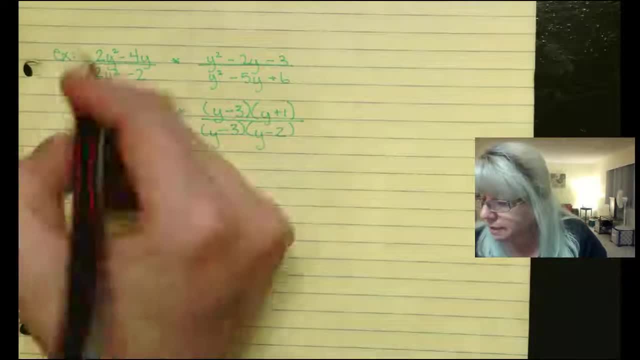 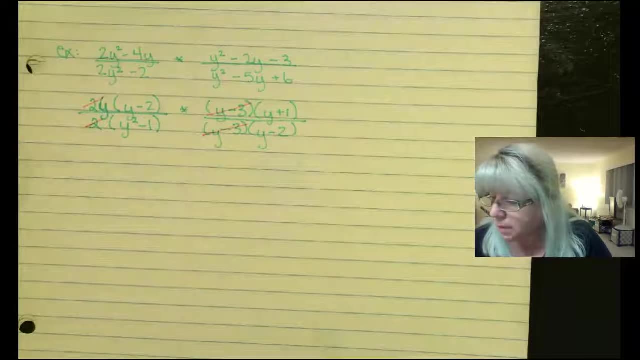 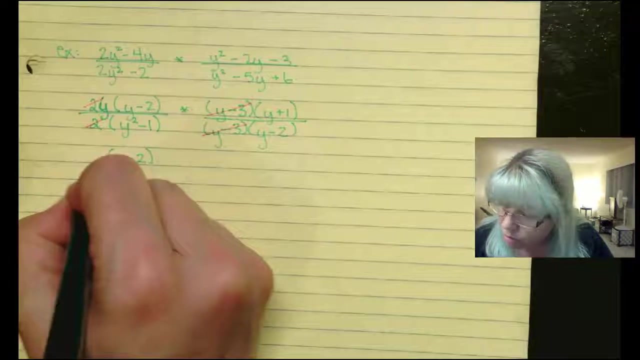 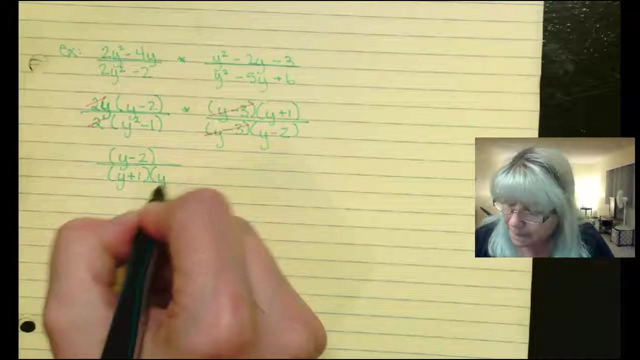 then carry it forward to see what happens. alright, Little steps: 2 over 2, that will go away, and the y minus 3 and the y minus 3 will go away. so let me rewrite what I have: Y minus 2 all over y, squared minus 1, can be factored y plus 1, y minus 1, times y. 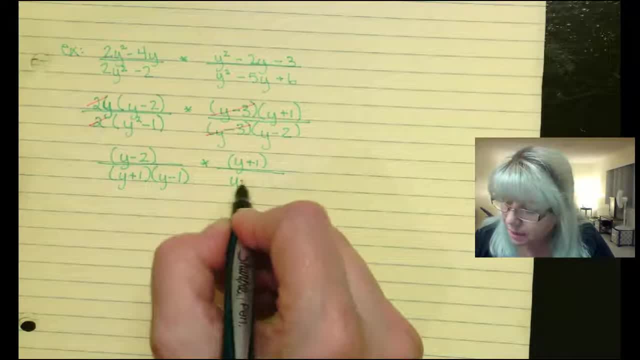 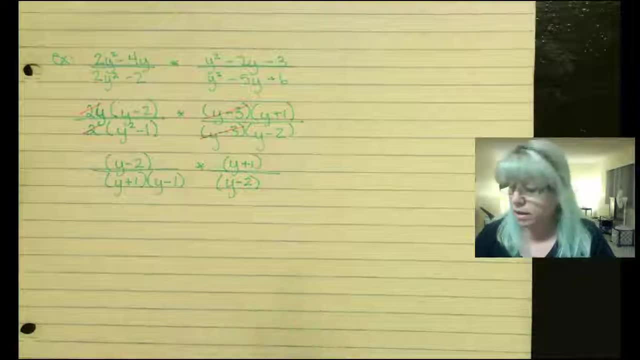 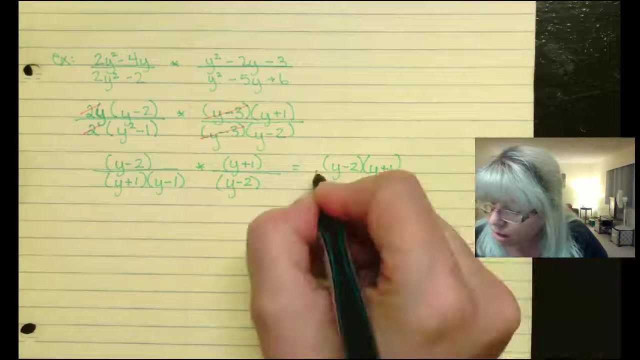 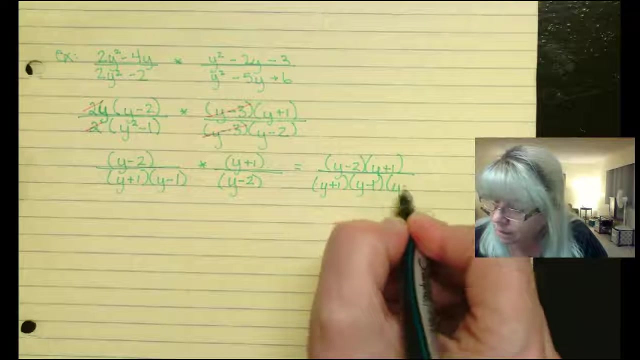 plus 1 over y minus 2, alright. Okay, There's still two separate fractions, but now I can put them as one fraction: Y minus 2 times. y plus 1 all over. y plus 1, y minus 1, y minus 2, alright. 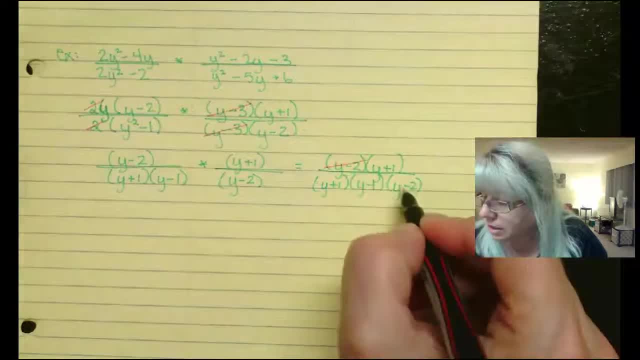 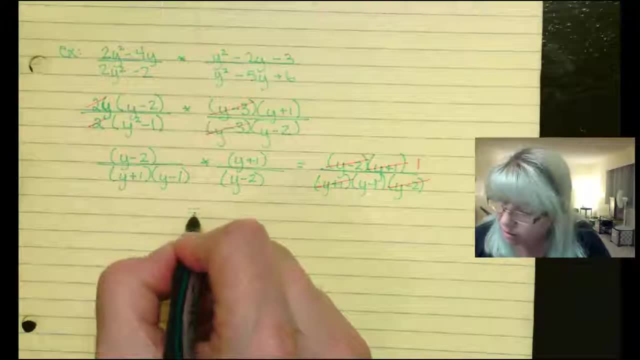 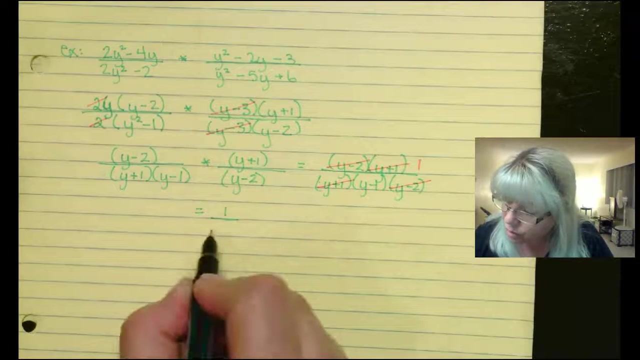 We can reduce again as it turns out: Y minus 2 and y plus 1.. There is a 1 still up there in the numerator. Okay, So the whole entire problem ends up reducing all the way down to 1 over y minus 1.. 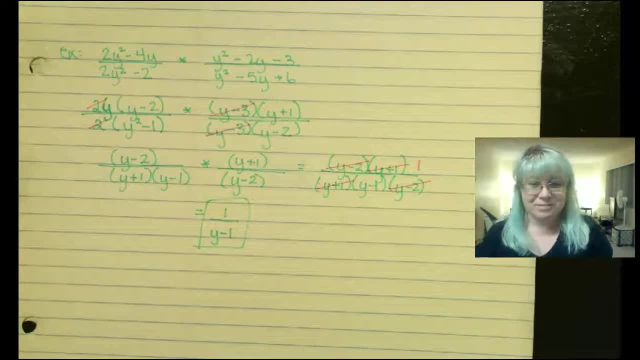 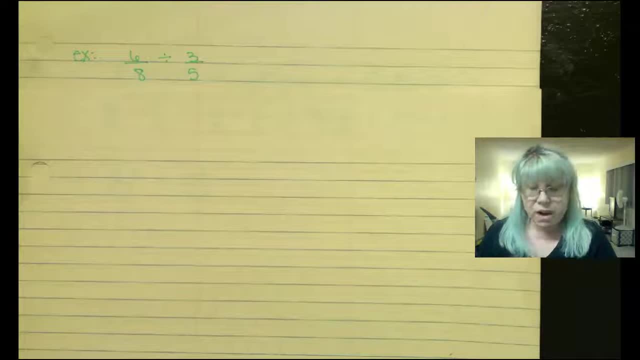 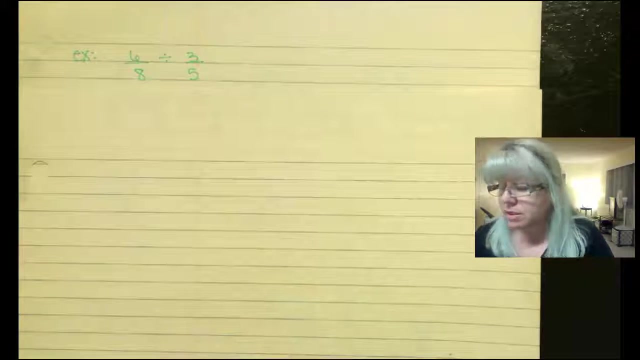 Okay, that was kind of cool, Alright, so let's deal with division now. Let's first start with division with fractions and then use that same process as in division of radical expressions as well as radical functions. Alright, So 6 eighths divided by 3 fifths. 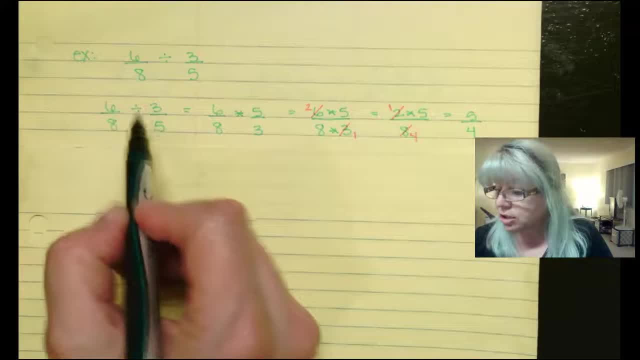 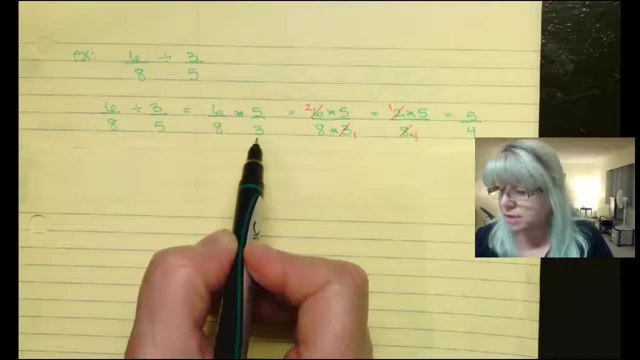 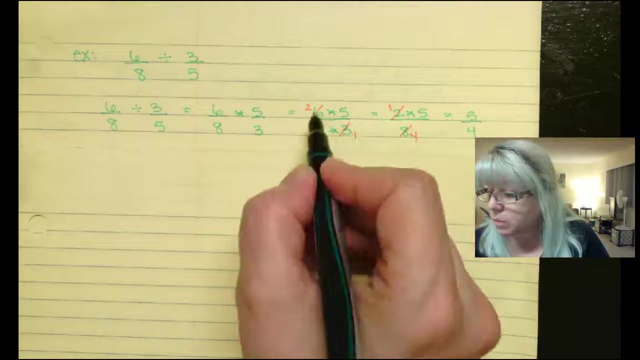 First thing I want to do is change the division by multiplication by the reciprocal. So now I have 6 eighths times 5 thirds. I can put it all under one fraction and reduce. 3 goes into 3 once, 3 goes into 6 twice, as well as 2 goes into 8 four times and 2 goes. 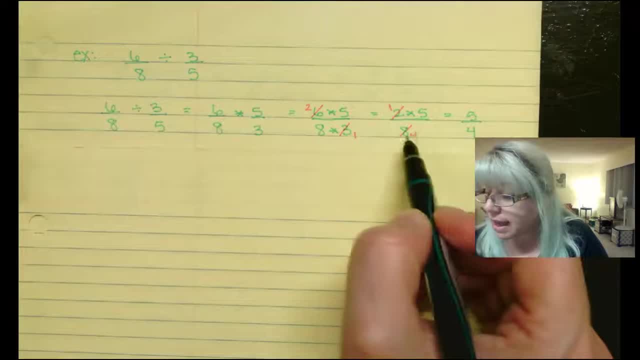 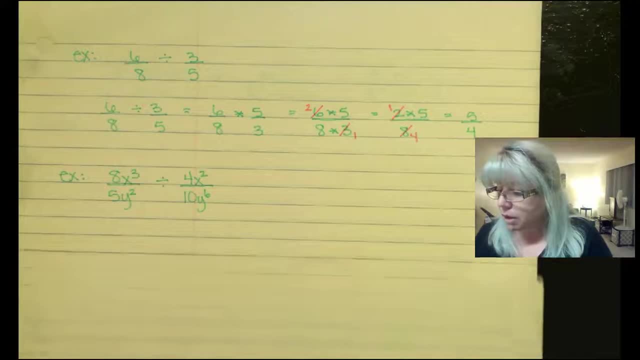 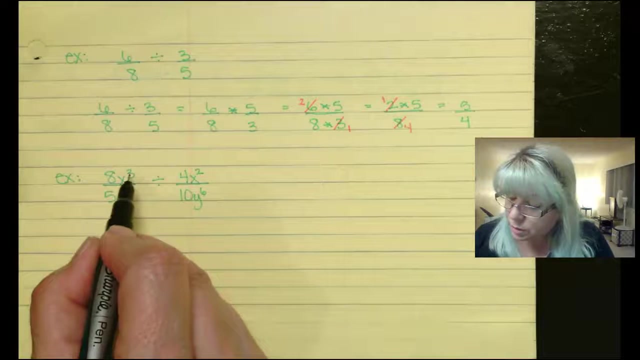 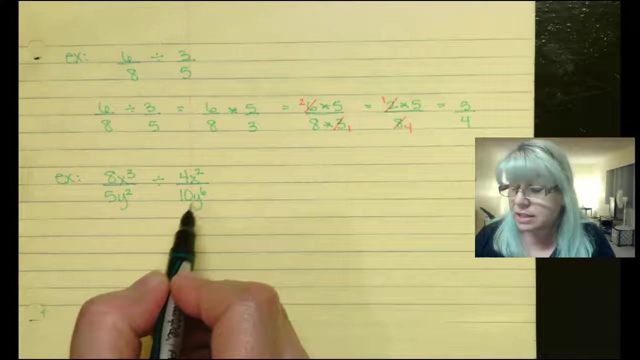 into 2. once, 1 times 5 is 5, and I'm left with a 4 in the denominator. So, following the same procedure, Alright. so let's try one with expressions: Alright, 8x cubed, all over 5y squared, divided by 4x squared, all over 10y to the sixth. 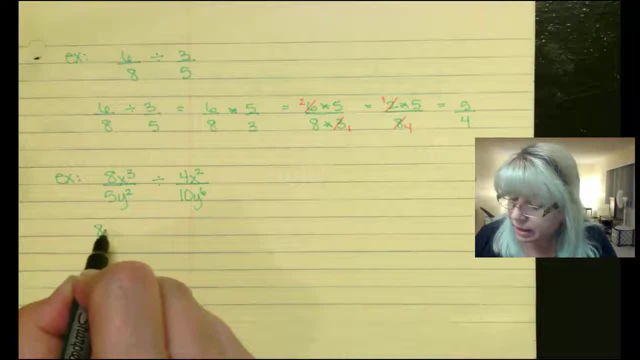 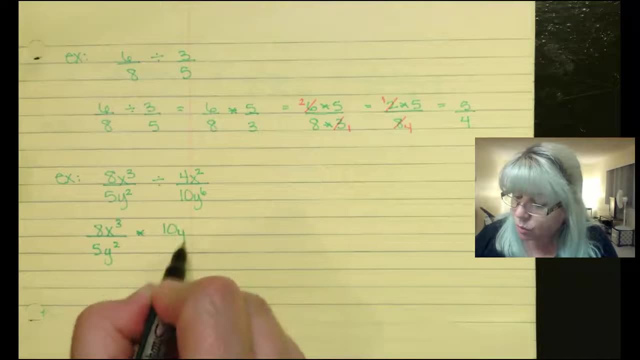 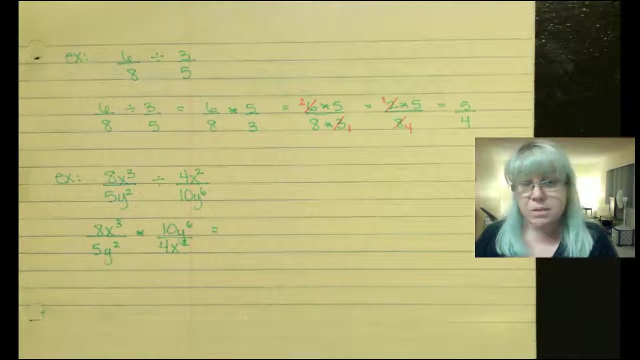 First thing I want to do is rewrite it as multiplication over 5y squared. Alright, Multiplication of the reciprocal 10y to the sixth, all over 4x squared. Now that I have that multiplication of the reciprocal, I'm going to combine them into. 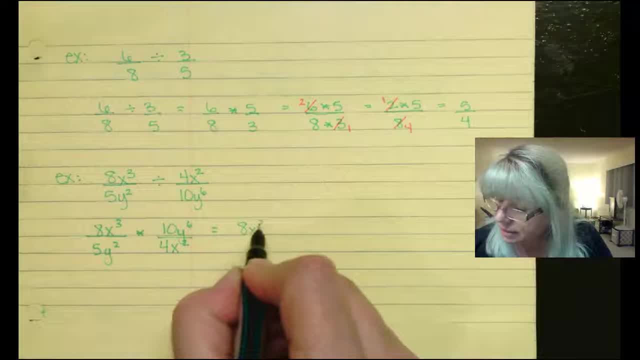 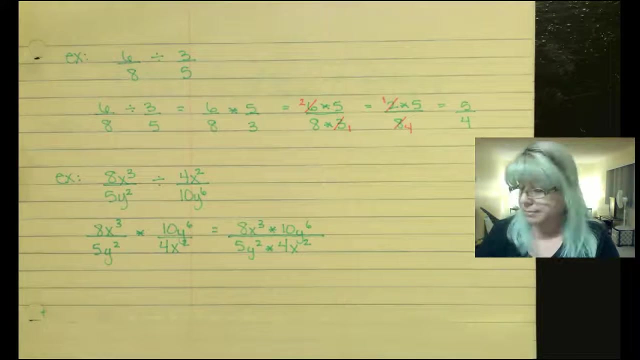 one fraction: 8x cubed times 10y to the sixth, All over 5y squared times 4x squared. Now I'm going to start reducing. 4 goes into 4 once. 4 goes into 8 twice. 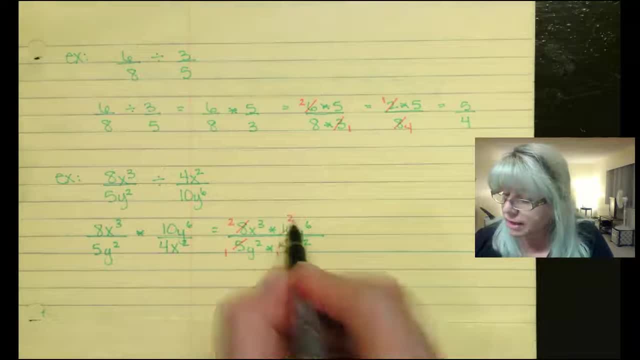 5 goes into 5 once, 5 goes into 10 twice. Just to clean it up, It's going to be 2 times 2 is 4.. x cubed y to the sixth, all over. Well, 1 times 1 is 1.. 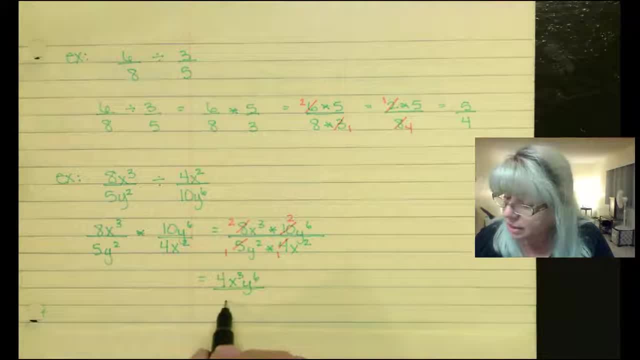 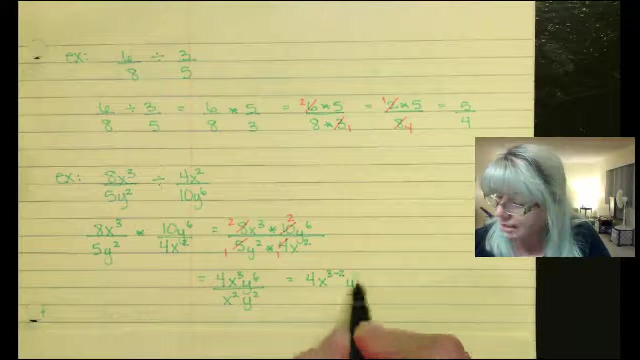 I don't need that in the denominator so I won't rewrite that. But it is x squared, y squared. Now I just need to deal with the exponents of the variables For x, 3 minus 2.. y, 6 minus 2.. 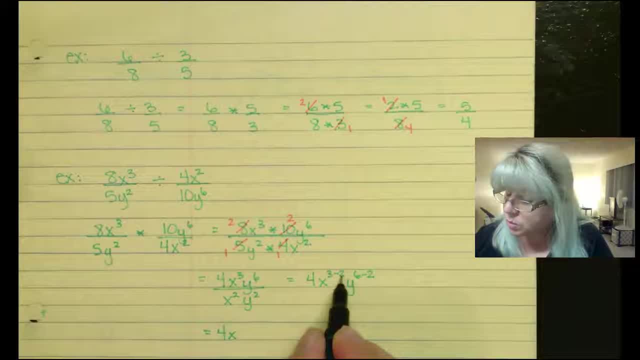 Therefore, 4, 3 minus 2 is 1, so it's x y. 6 minus 2 is 4.. y to the fourth. There we go. All right, let's work with a little bit more complex problem. 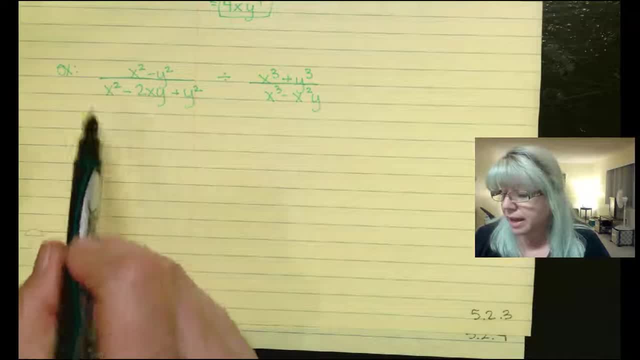 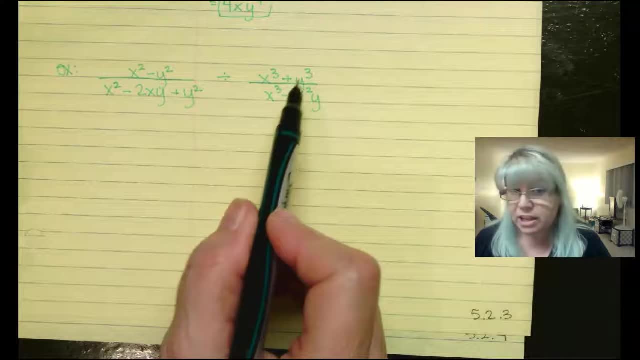 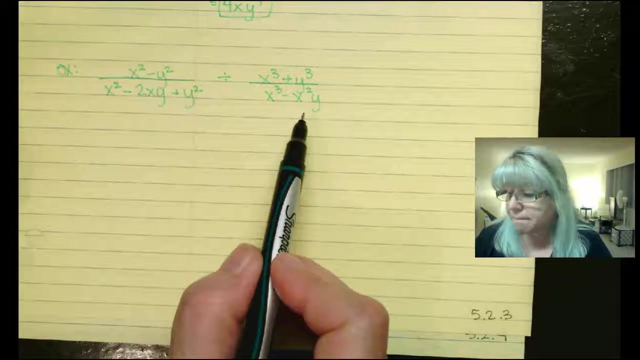 x squared minus y squared all over x squared minus 2xy plus y squared divided by x cubed plus y cubed all over x cubed minus x squared y. All right, First thing I'm going to do here is I'm going to multiply. 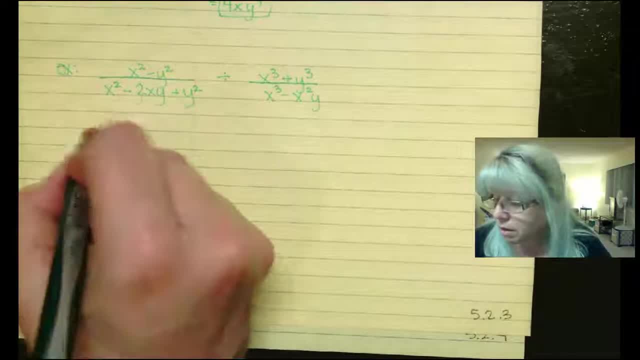 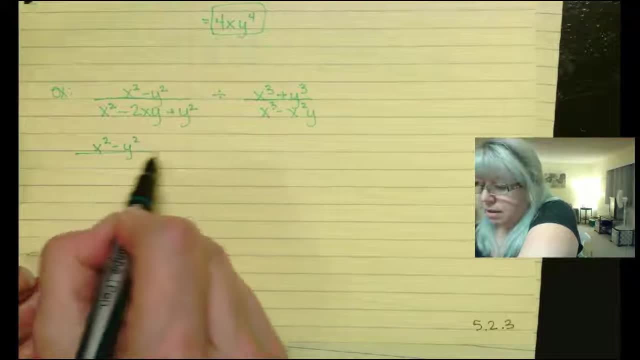 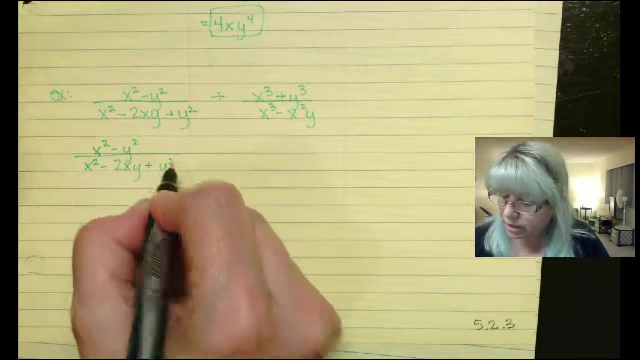 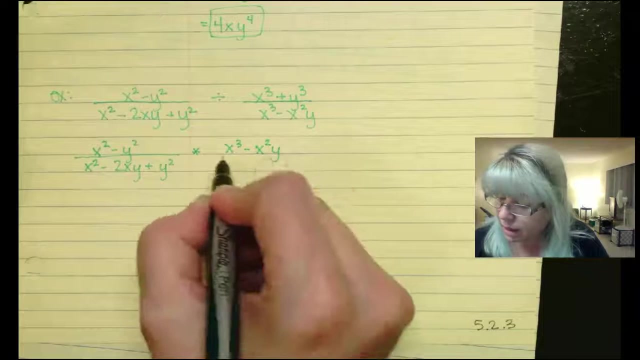 I'm going to multiply by the reciprocal: All right, x squared minus y squared. Oops, sorry about that. All over x squared minus 2xy plus y squared times. x cubed minus x squared y. All over x squared minus y squared plus y cubed. 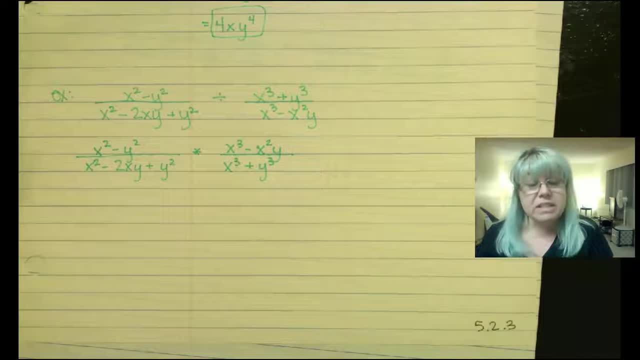 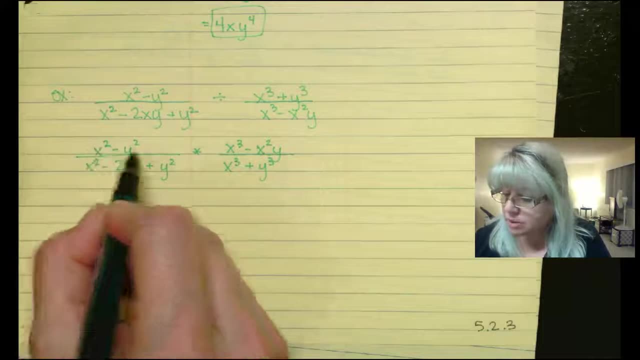 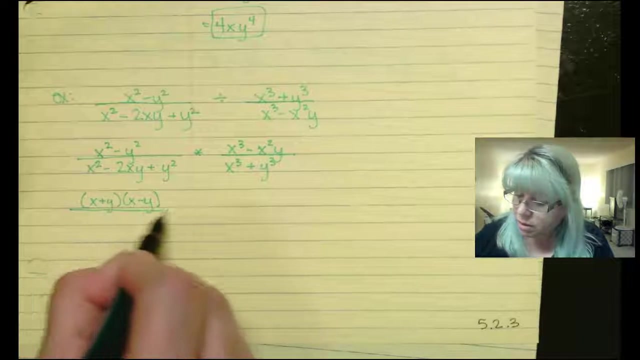 Okay, Now that I have it rewritten, I'm going to factor each numerator and each denominator, if I can. All right, x squared minus y squared is going to be x plus y, x minus y, x squared minus 2xy plus y squared. 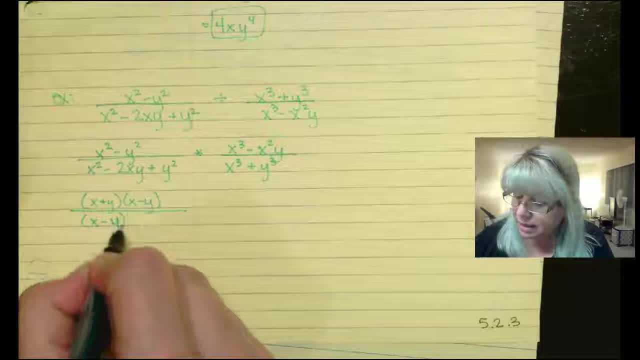 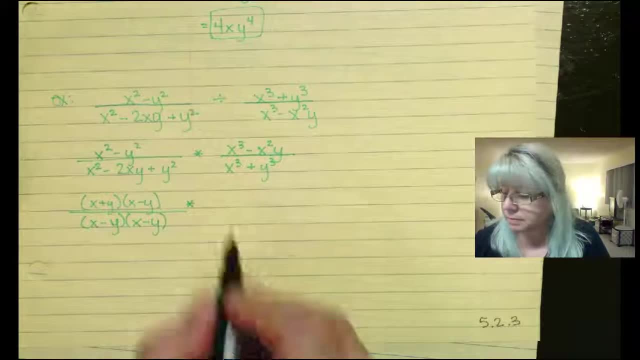 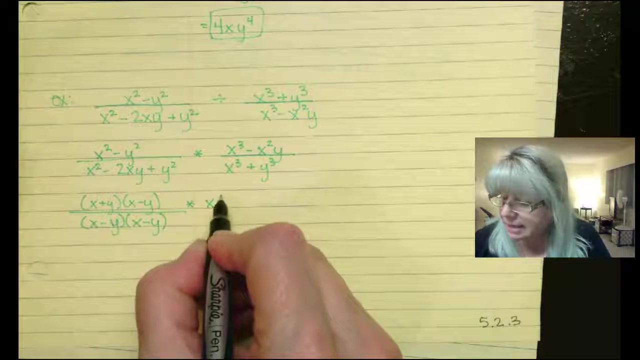 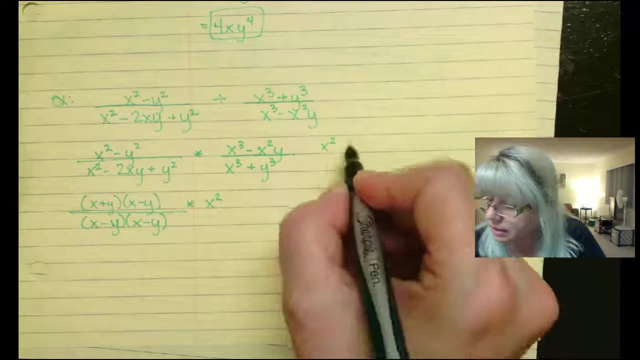 It's going to be x minus y times, x minus y times, Just keeping them separate for now. I'm going to squish them together in a second. I can do an x and that would leave x squared. I can actually pull out an x squared, leaving x minus y. 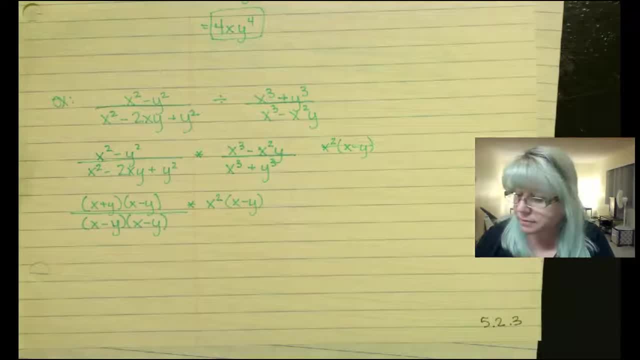 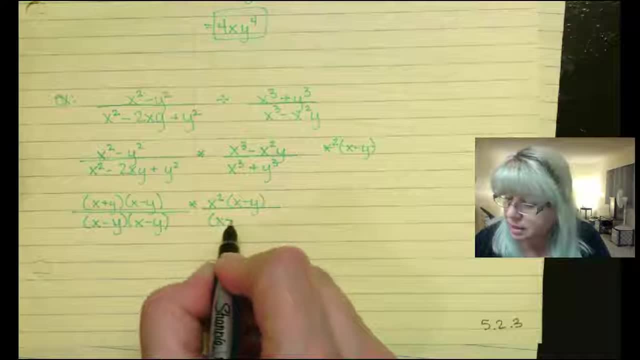 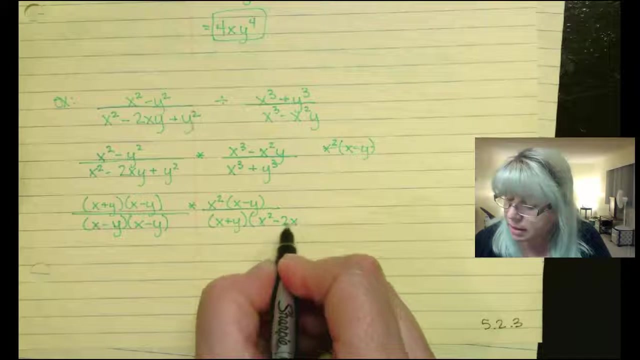 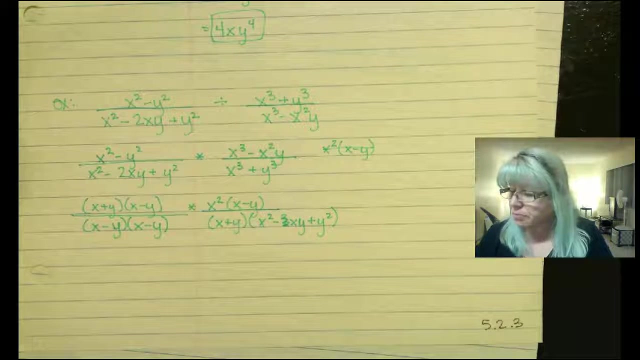 All right, It's just kind of my workspace right there. Then x cubed plus y cubed is a perfect cube. That's going to be x plus y times x squared minus 2 minus xy plus y squared. Sorry about that, Okay. 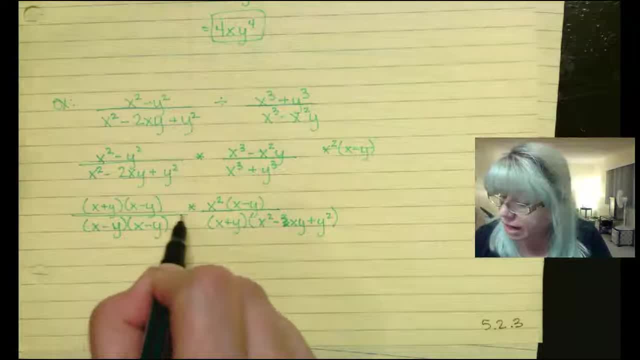 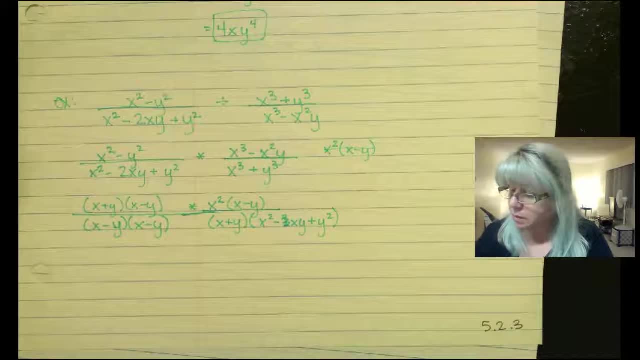 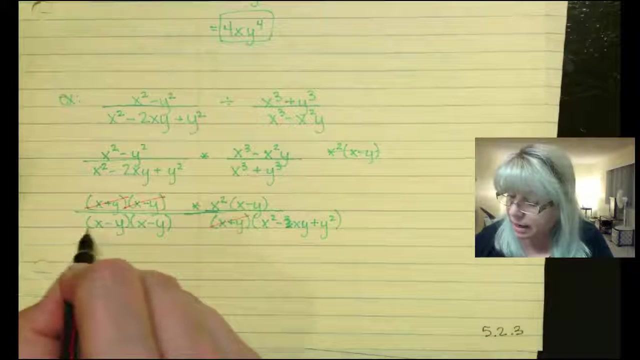 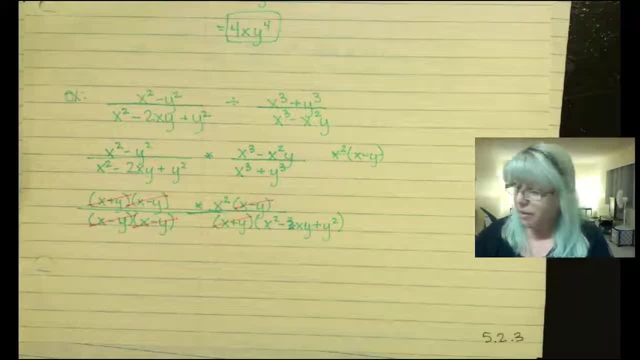 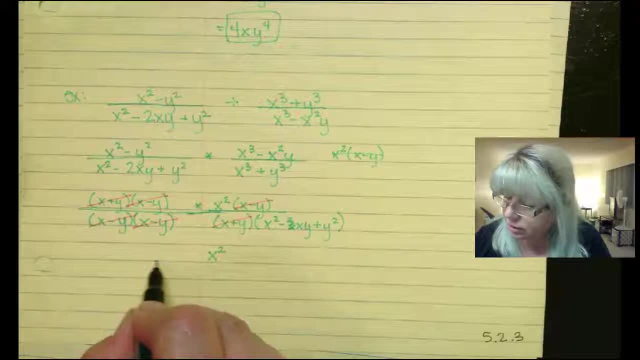 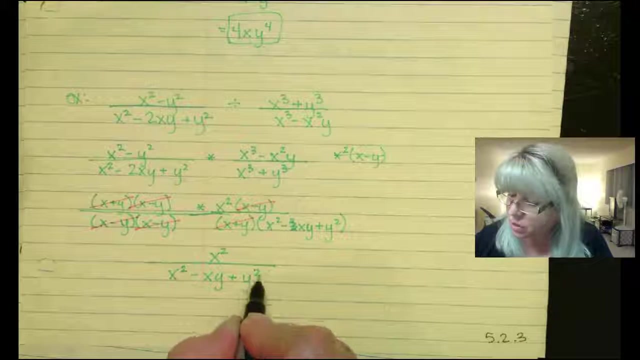 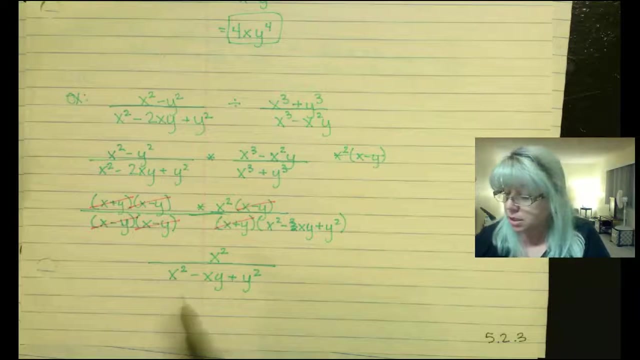 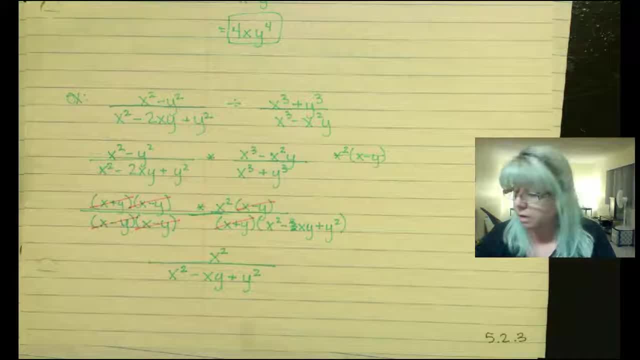 but keep in mind I cannot do that. We cannot do that because we cannot cross the subtraction and addition. These are three terms in the bottom and one term on the top. I cannot cross this subtraction and addition. So that is my final answer. 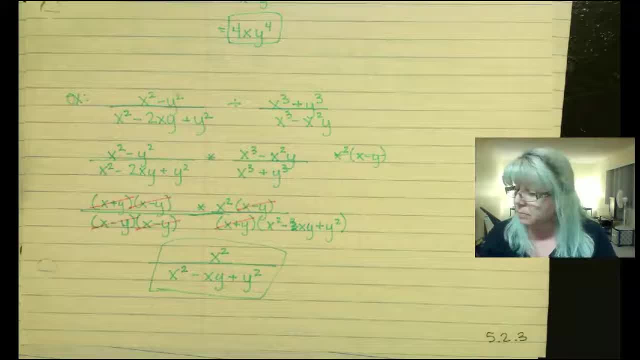 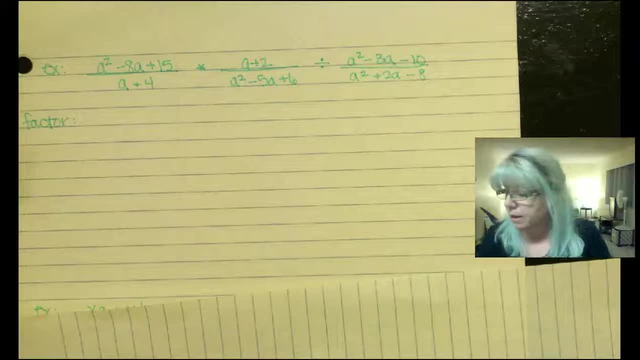 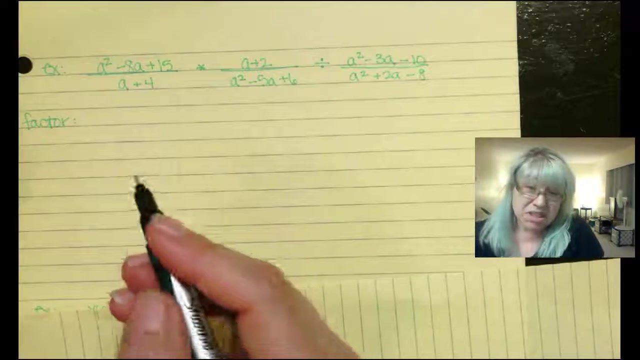 It is as reduced as I can get it. All right, Let's throw the kitchen sink at you here. Okay, I have multiplication and I have division. So the first thing I'm going to do- personally I'm going to do- is I'm going to go ahead and factor each numerator and denominator. 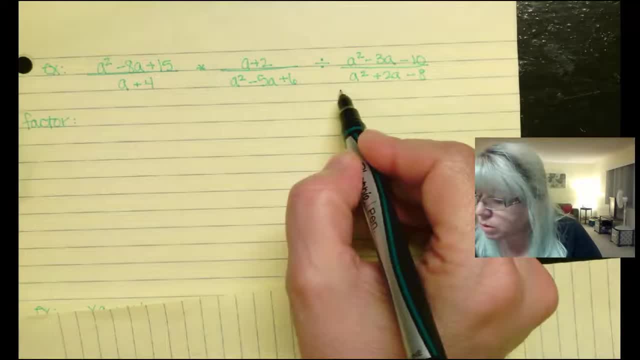 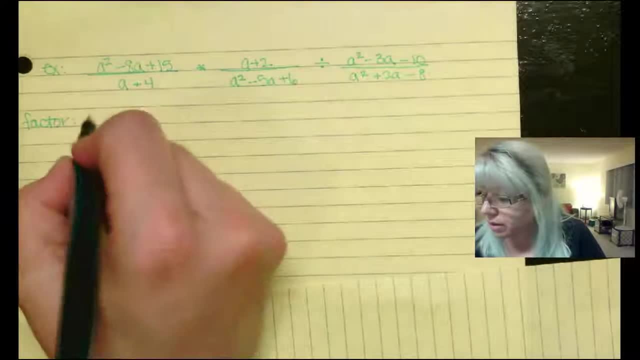 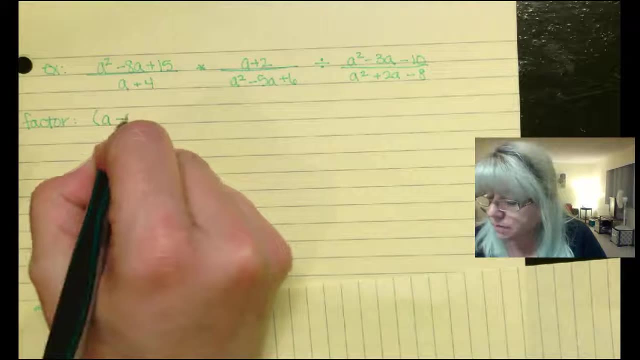 And while I'm doing that, I am going to multiply, change this to multiplication of the reciprocal. So first let's just figure out all the factors. All right, a squared minus 8a plus 15.. It's going to be a minus 5, a minus 3,. 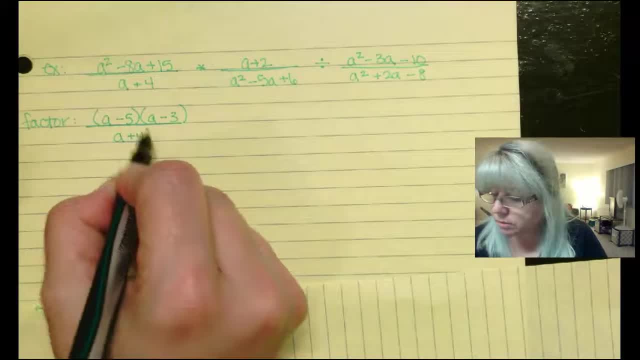 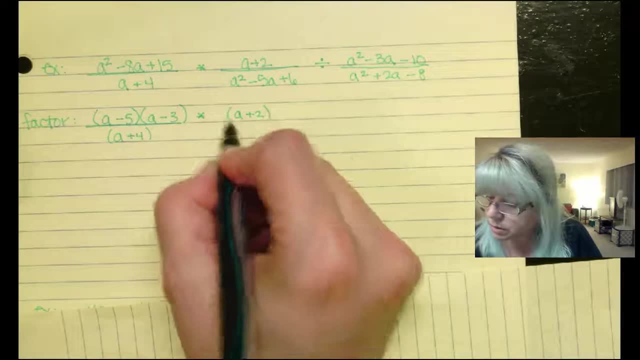 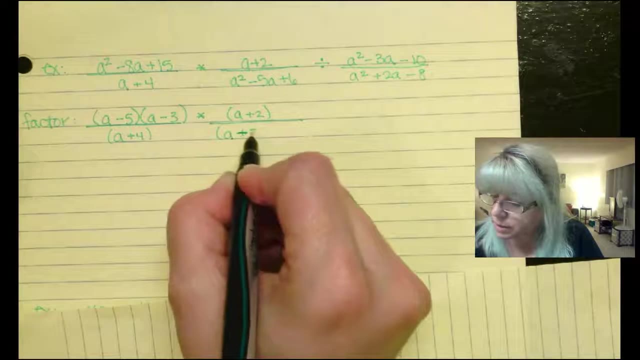 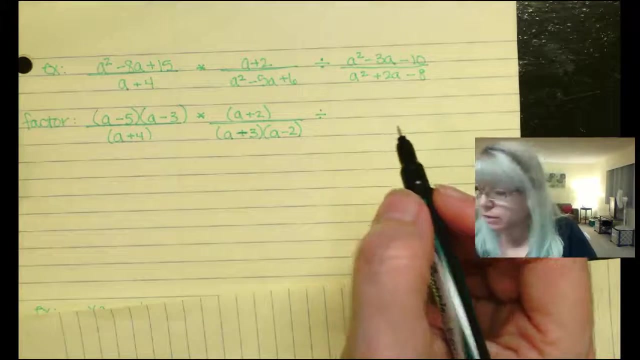 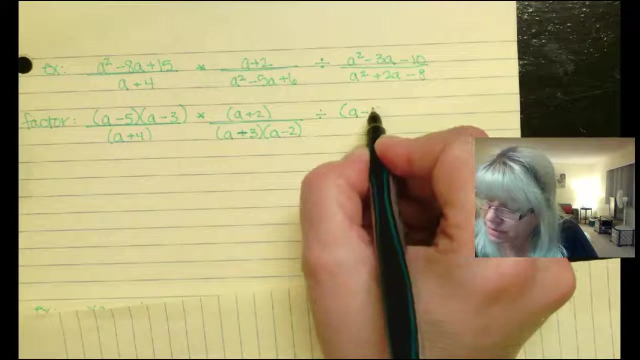 all over a plus 4, times a plus 2,. all over a plus- oops- minus 3a minus 2, divided by- and I'm just going to factor everything first- a minus 5a plus 2,. 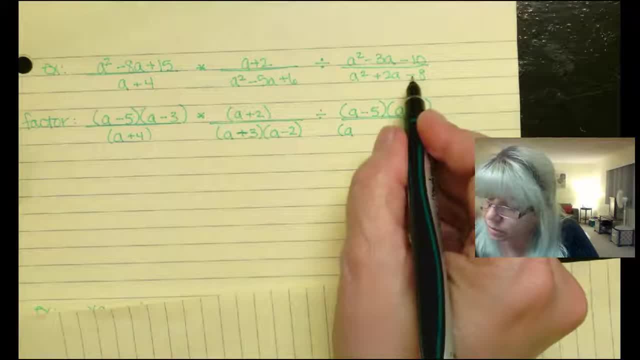 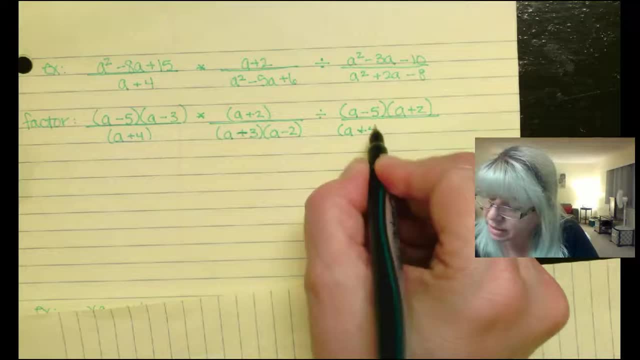 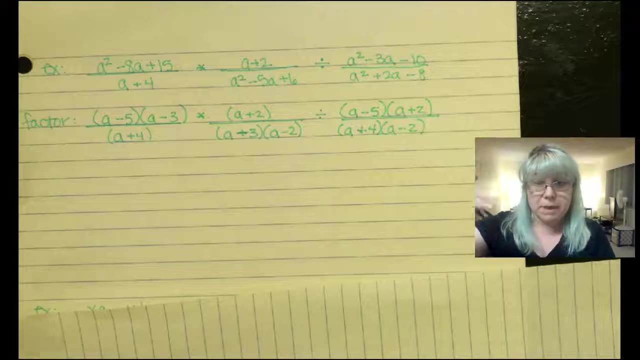 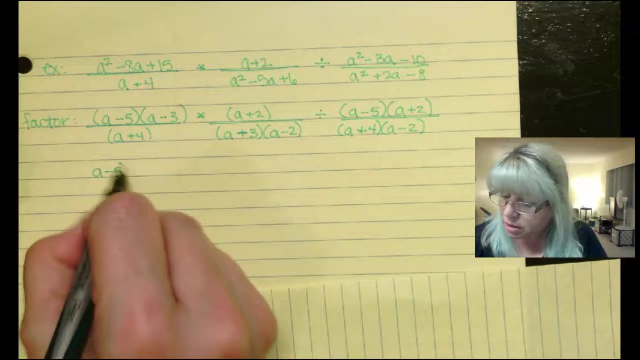 all over. right, that's got to be 4 and 2, where 4 is the positive. There we go. Okay, One last thing. I'm going to multiply by the reciprocal of this third term and put it all under one fraction. 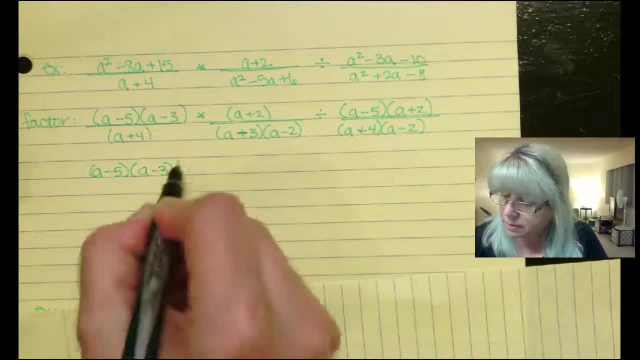 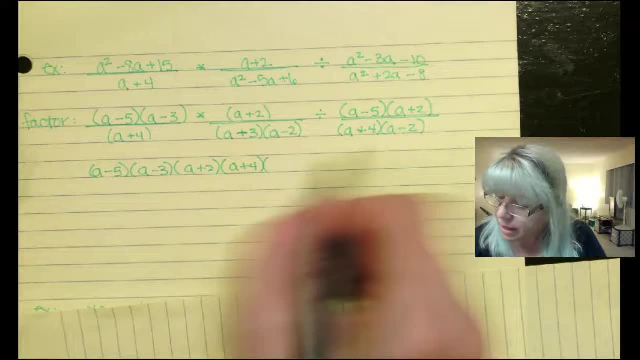 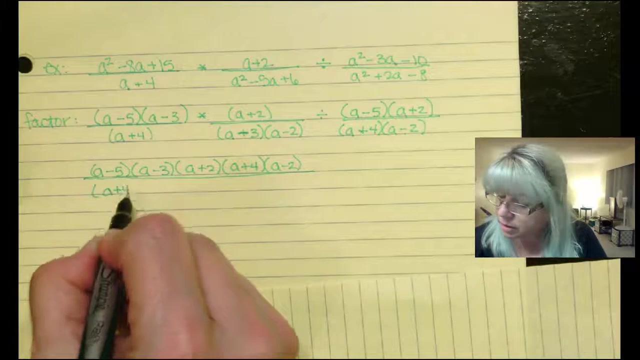 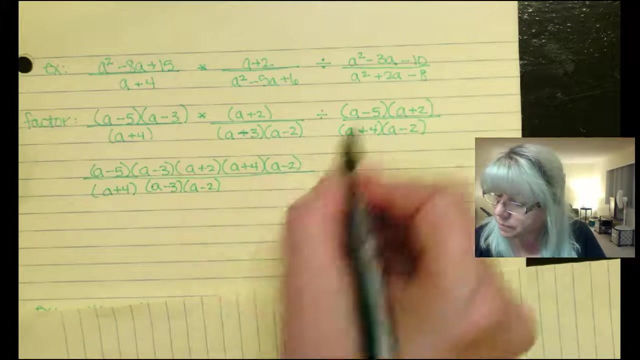 a to the minus 5, a minus 3, a plus 2,, all over a plus 4, a minus 2,, all over a plus 4, a minus 3, a minus 2, a minus 5,. 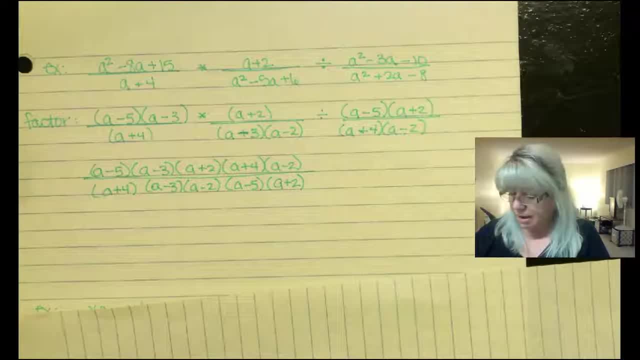 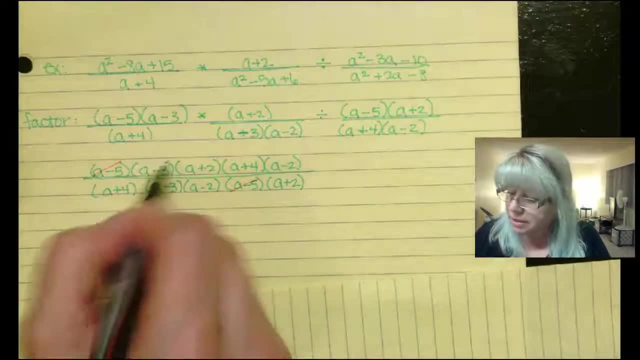 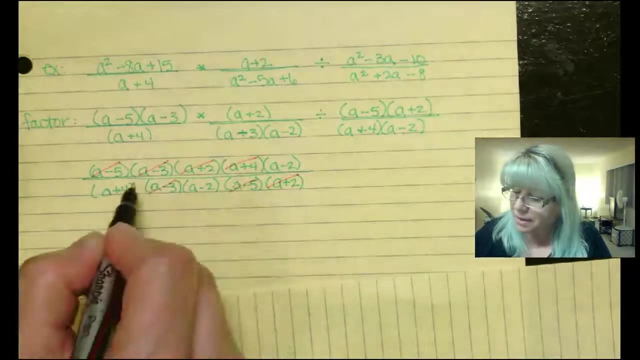 a plus 2.. All right, Now it's time to reduce: a minus 5, a minus 5, a minus 3, a minus 3, a plus 2, a plus 2, a plus 4, a plus 4,. 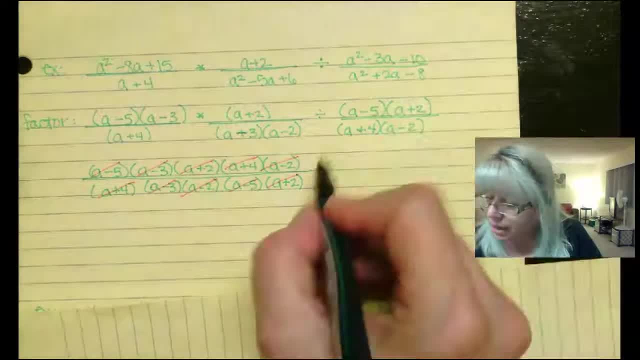 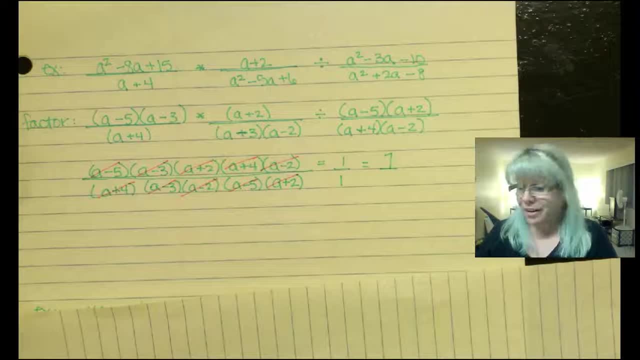 a minus 2, a minus 2.. This whole thing is a 1 over a 1,, which is a 1.. Wow, A lot of work for just one. Kind of cool too that that ended up. it looked like a big fat mess in the beginning. 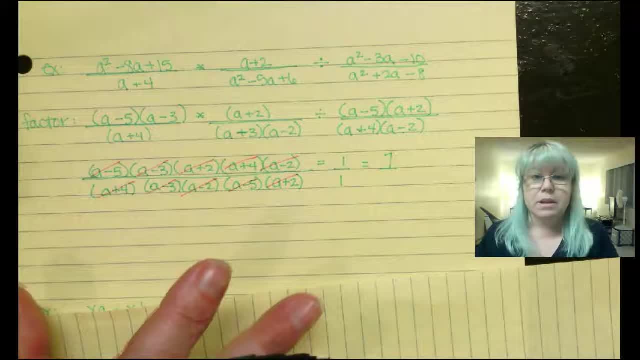 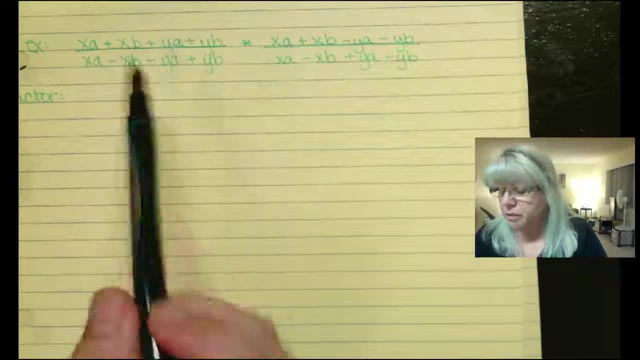 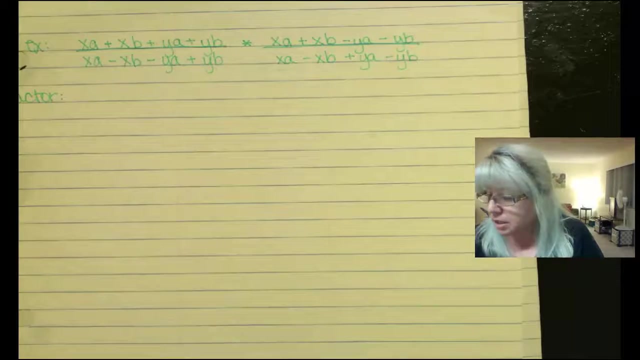 but it all all ended up multiplying to 1. Kind of cool. All right, Let's try another problem. Generally, when we have four terms, you're going to use grouping to factor, So let's go ahead and group. I'm going to just go ahead and group it kind of as it sits. 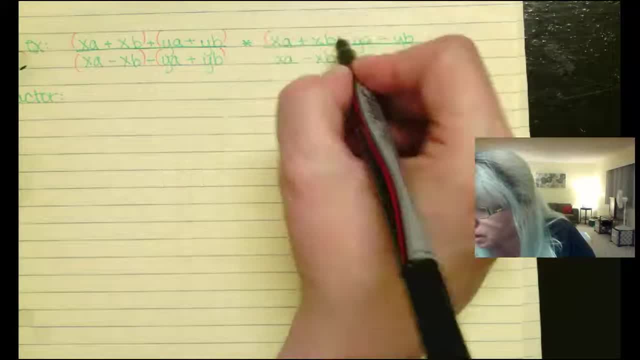 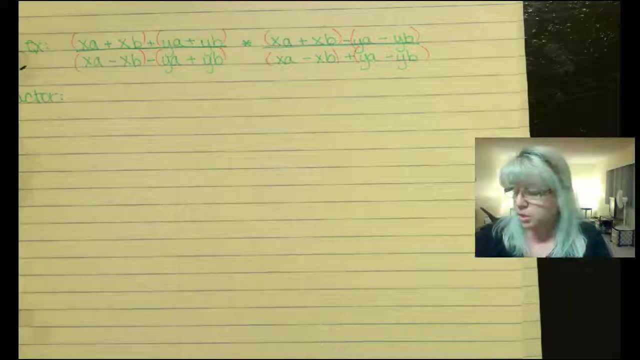 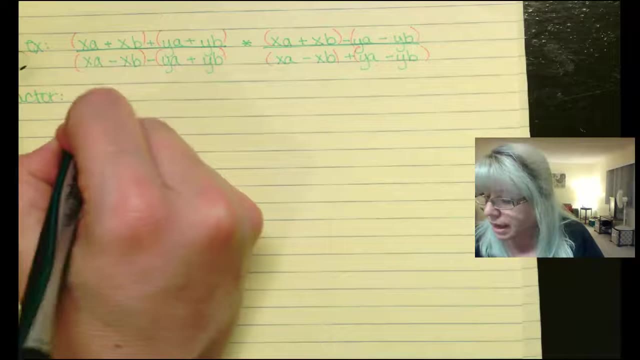 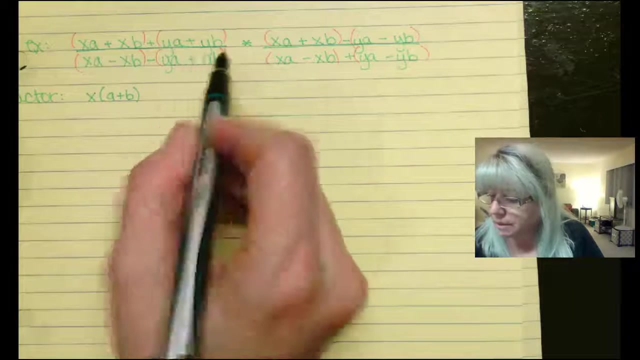 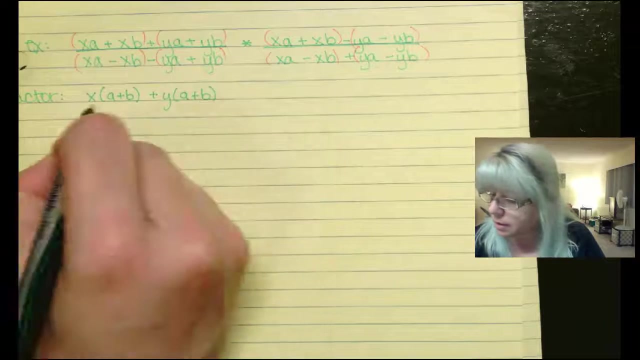 I'm thinking of grouping it into two. I'm not quite aligning it perfectly with the signs, I'm just kind of thinking of them in groups of two. So x a plus x b will factor into x times a plus b. y a plus y b will factor to y a plus b. 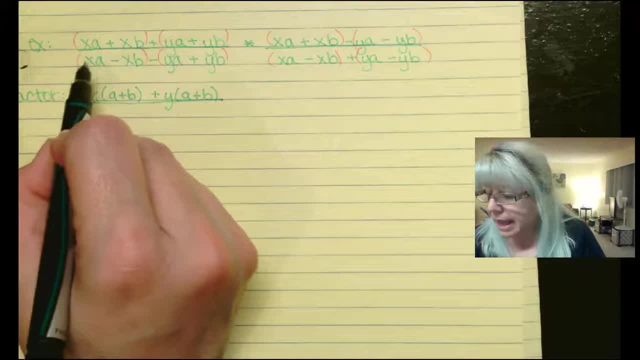 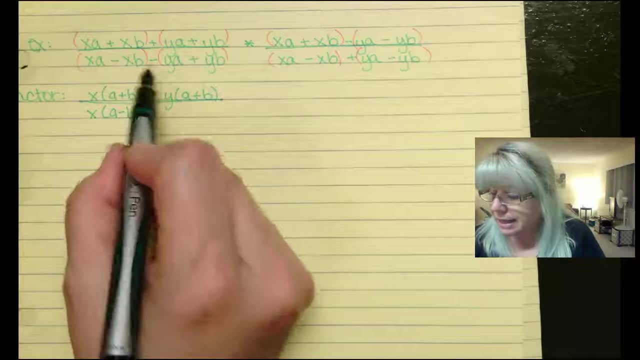 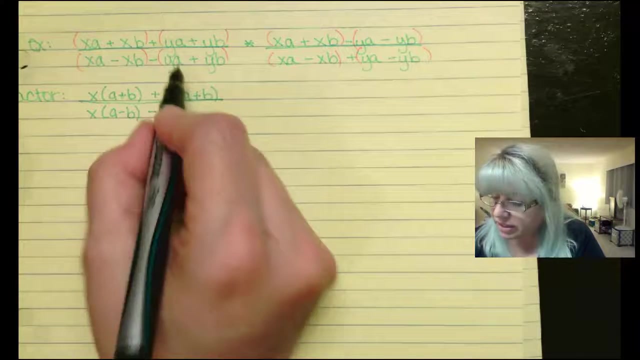 All right. Denominator: x a minus x b will be x a minus b. Negative y a plus y b. I can factor out that negative y, That will leave me a and negative b, because negative times a negative will be that positive, right there. 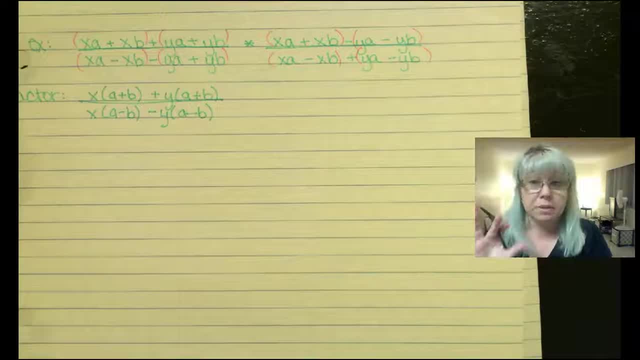 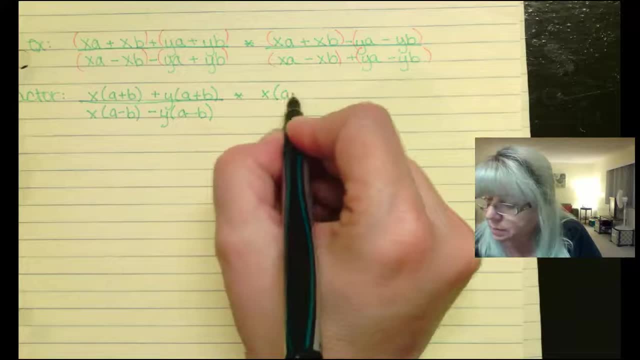 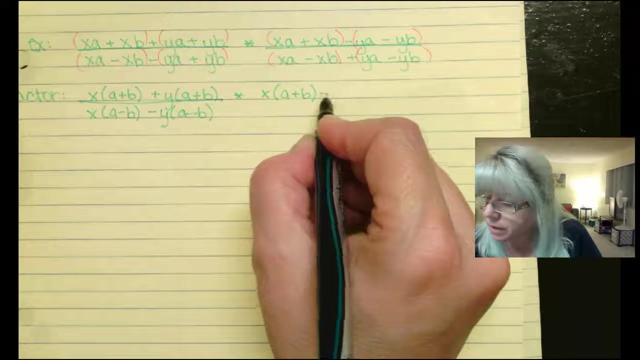 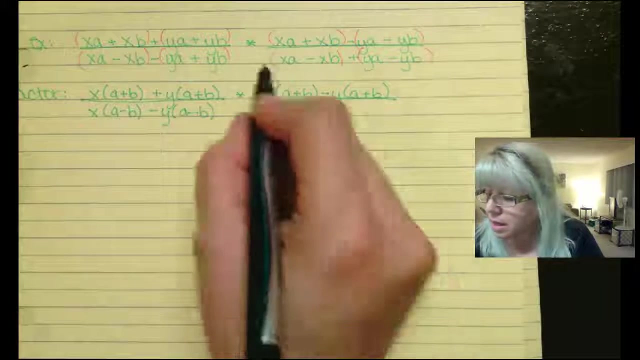 Minus b. So the first term is factored Times. All right, X a plus b. Let's go ahead and factor out a minus y. out of here Minus y, leaving me a plus b. All right Denominator will be x a minus b. 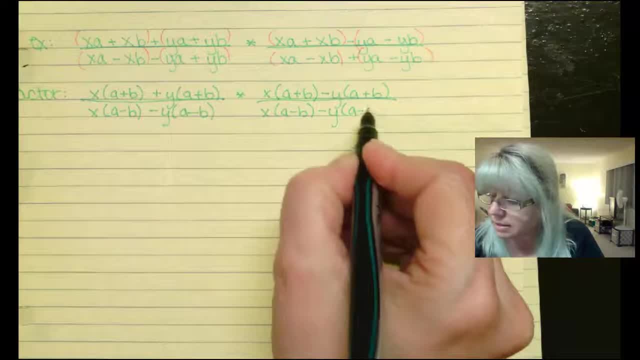 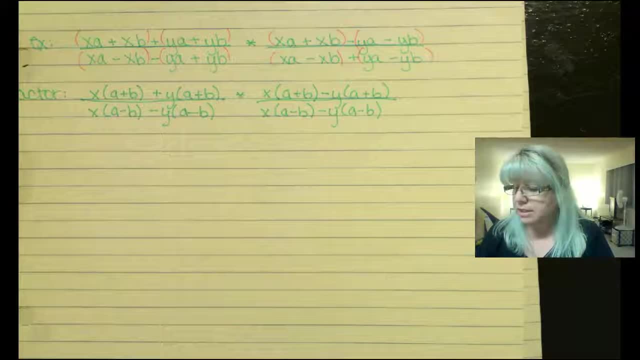 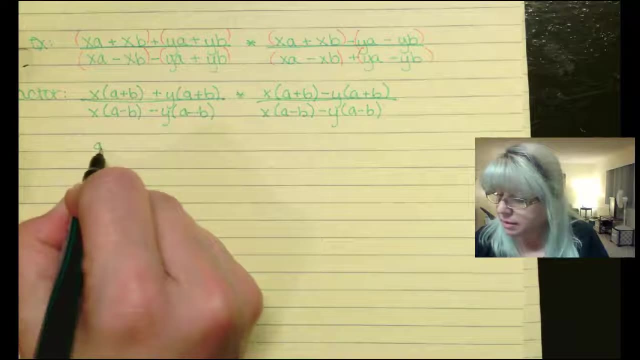 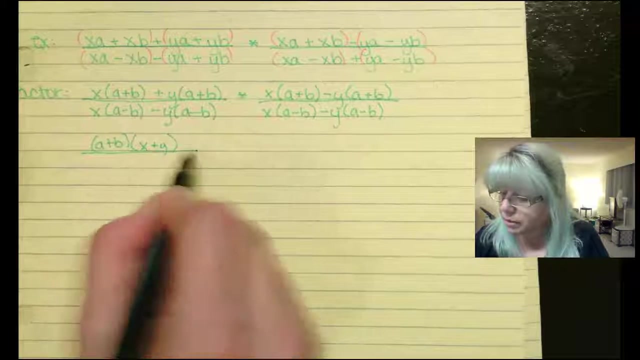 And we can factor out a negative y, again A minus b. All right, One more step to factoring X plus y. Let's factor out this: a plus b, X plus y, All over: A minus b, X minus y. 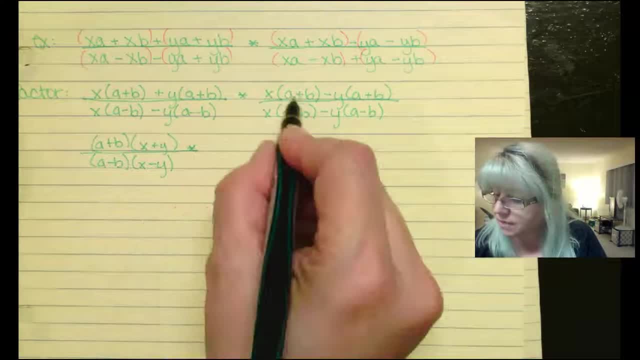 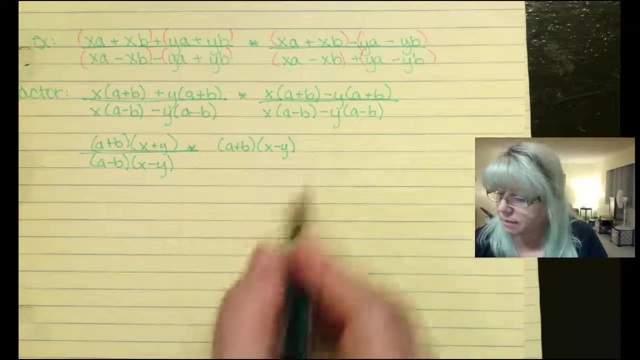 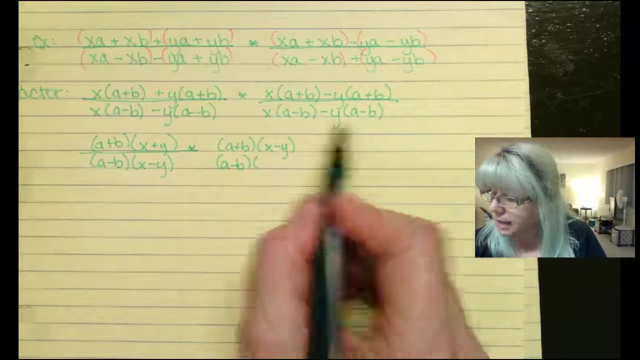 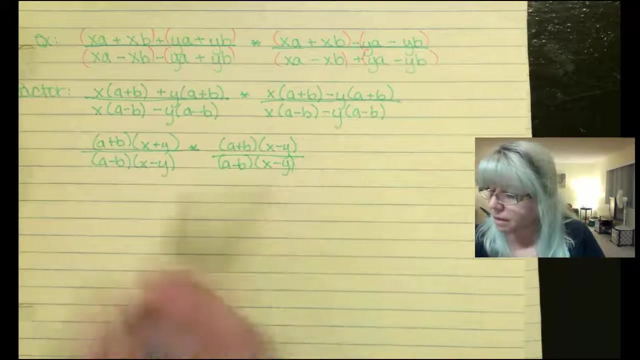 Times X minus y. Or let's factor out the a plus b And the x minus y, Factor out the a minus b, Leaving behind X minus y. Just want to check my work here. Okay, If I factor out a negative y. 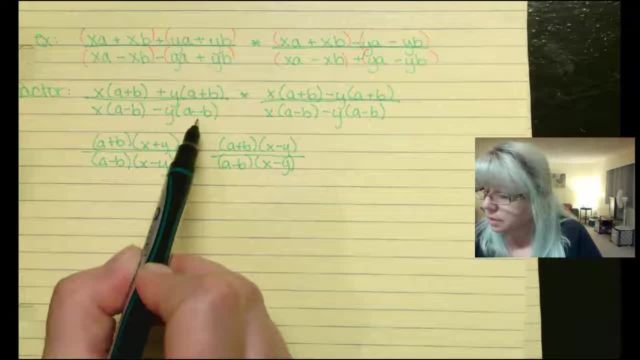 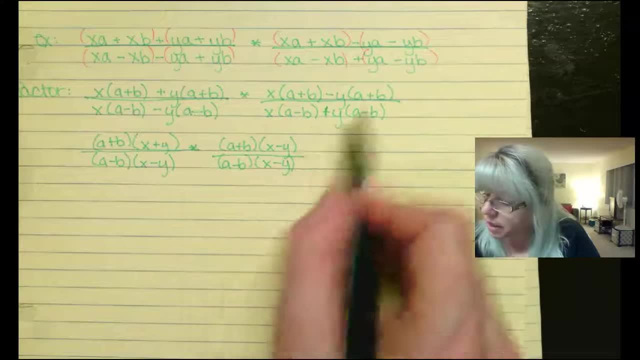 That's going to be Yeah, Negative b. That makes sense And I just want to make sure. Oh, I should have factored out just a y, Positive y. There we go. Thought something looked weird there. Okay, Found my mistake. 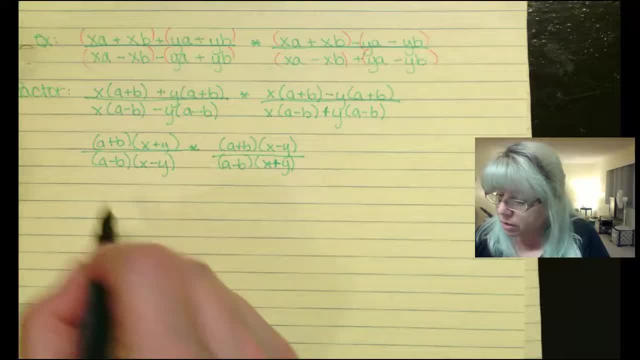 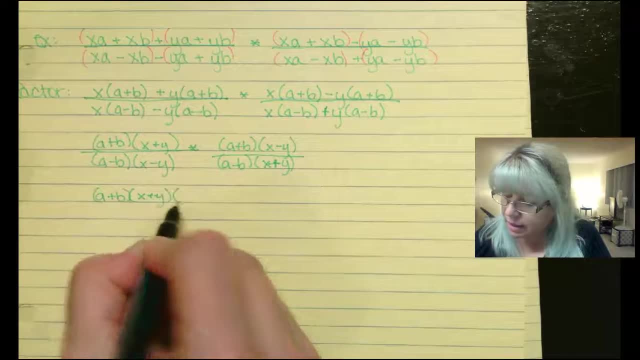 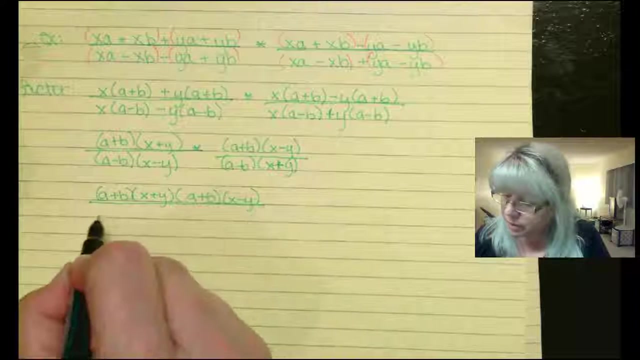 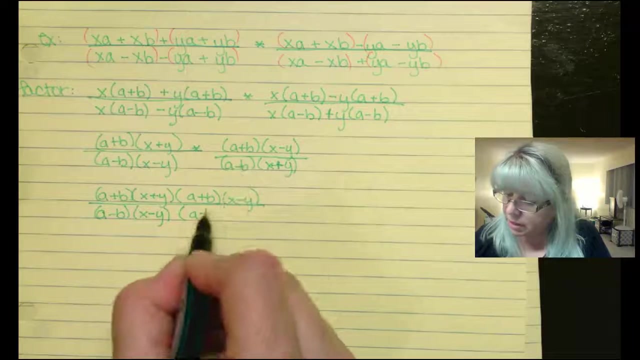 Yay, All right, This is all going to be on one fraction: A plus b, X plus y, A plus b, X minus y, X minus y. All over: A minus b, X minus y, A minus b. 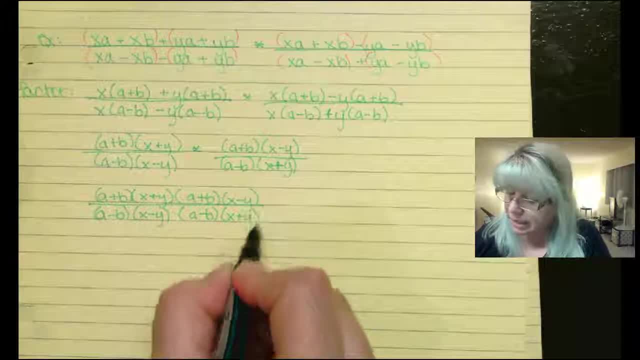 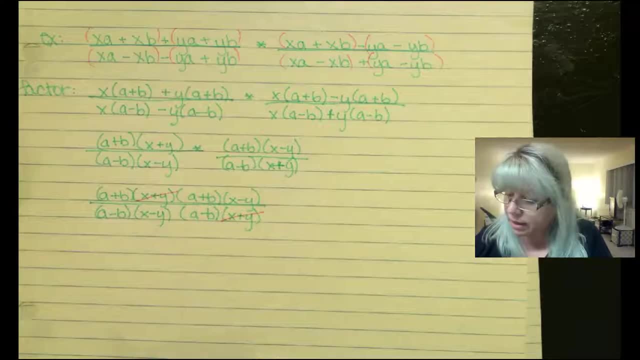 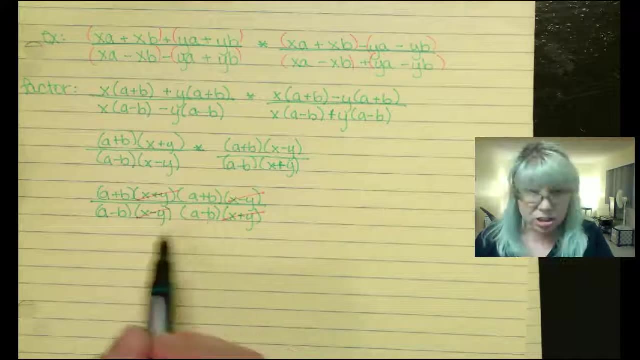 X plus y. Is there anything that we can cancel Or is there anything we can reduce? Yes, X plus y, X plus y, X minus y, X minus y. I cannot do a plus b And a minus b. That just won't work. 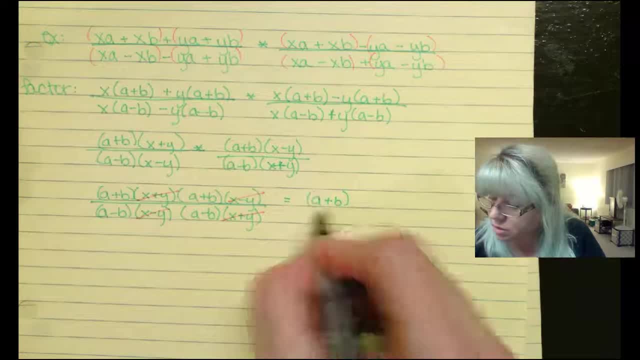 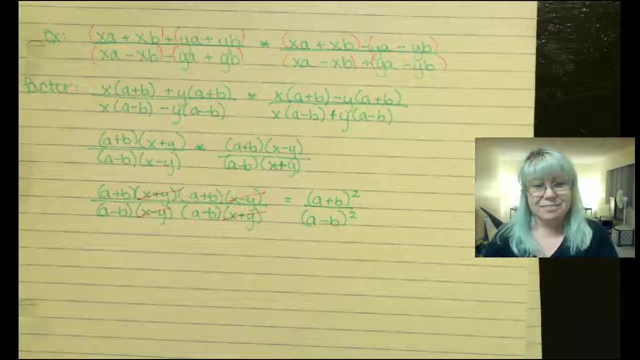 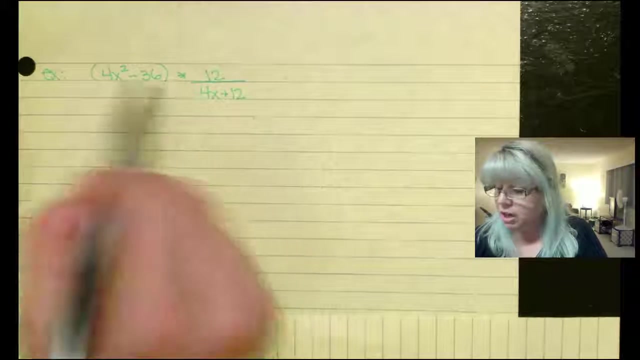 So my answer: A plus b Squared Over A minus b Squared. That's my final answer. Let's do a couple more examples. Okay, Before I do any multiplication, I'm going to factor This expression: 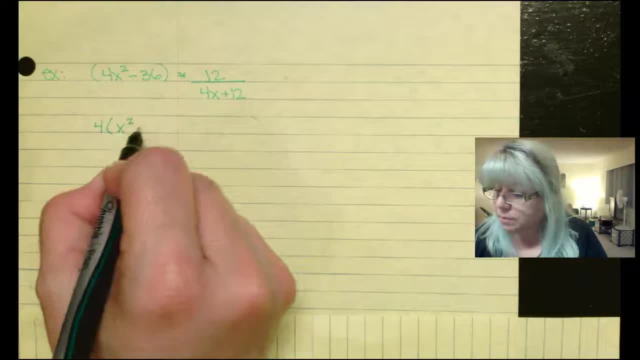 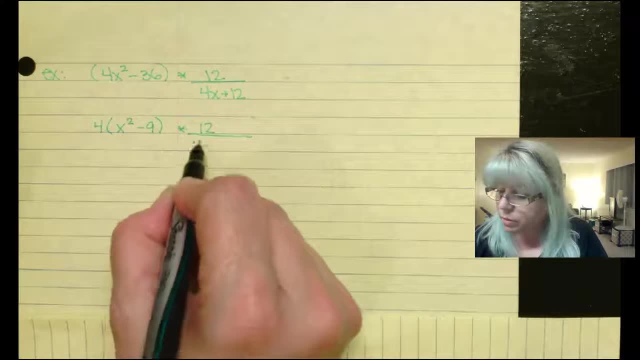 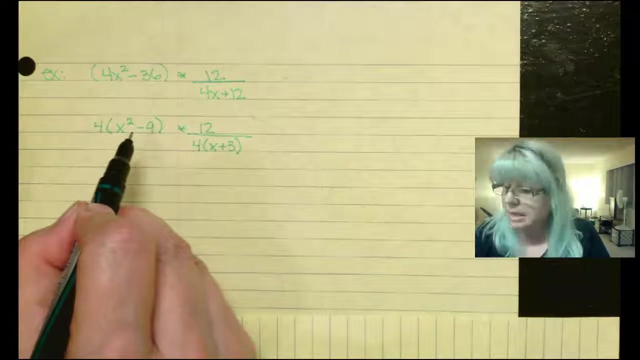 And pull out a four X squared Minus nine Times twelve. I'm going to factor the denominator Four X plus three For the x Squared Minus nine. I can factor that as well. So it's going to be four. 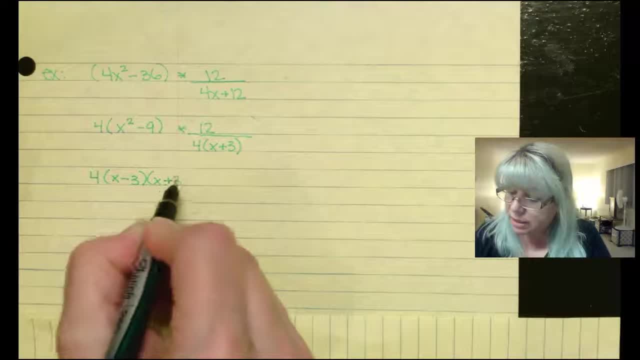 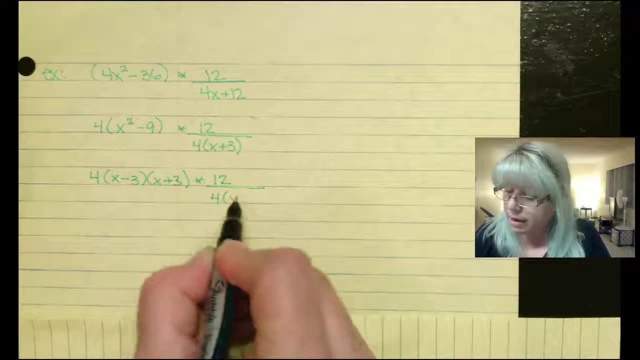 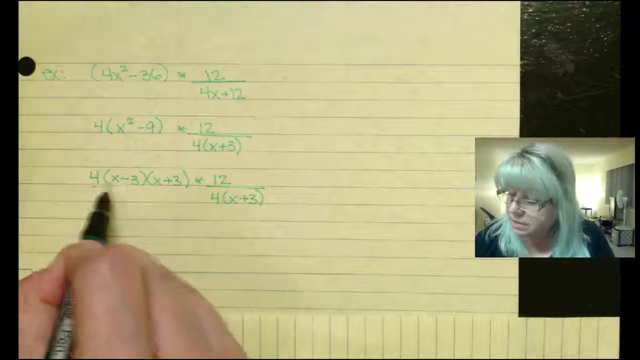 X minus three, X plus three Times Twelve Over Four X plus three. Now I'm going to go ahead and combine it. I can say that there is a one underneath here, So that's going to be Four. 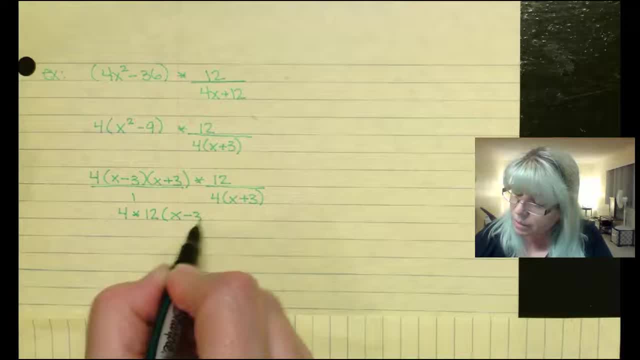 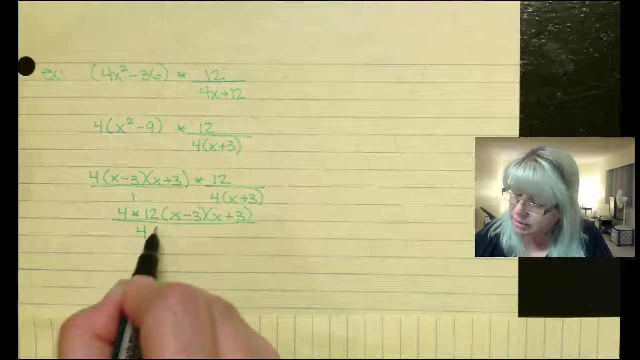 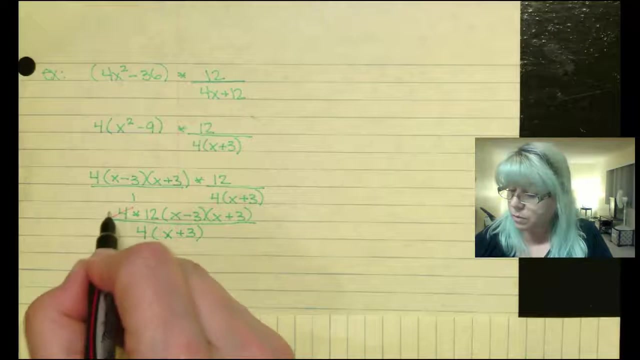 Times twelve Times x minus three, X plus three, All over Four Times x Plus three. Now I can reduce: Four goes into four once Four goes into four. once X plus three goes into x plus three. once X plus three goes into x plus three once. 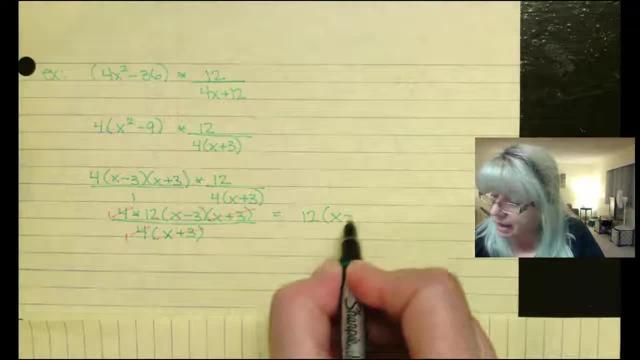 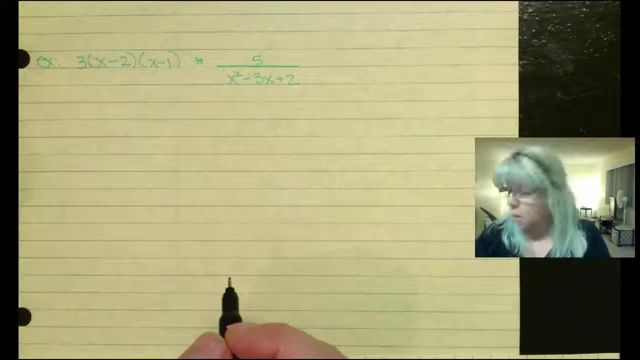 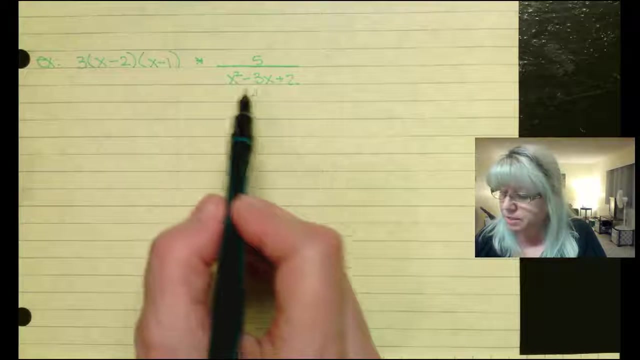 Leaving Twelve X minus Three. Not so bad, Not so bad, All right. Similar problem, But actually the first term is already factored, So the only thing that I need to factor is this: x squared minus three, x plus two. 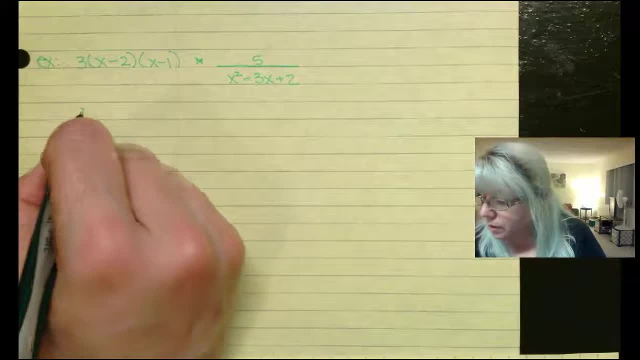 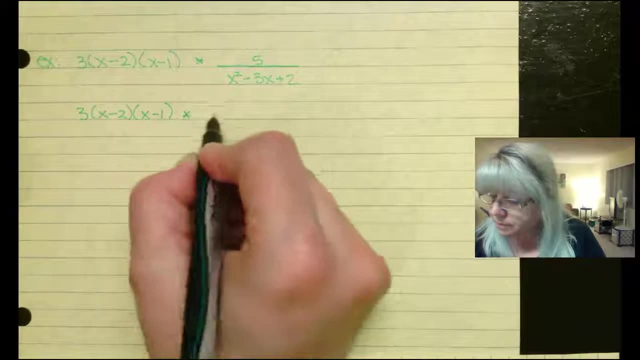 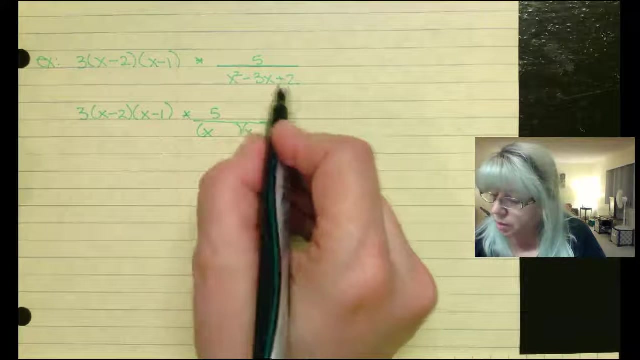 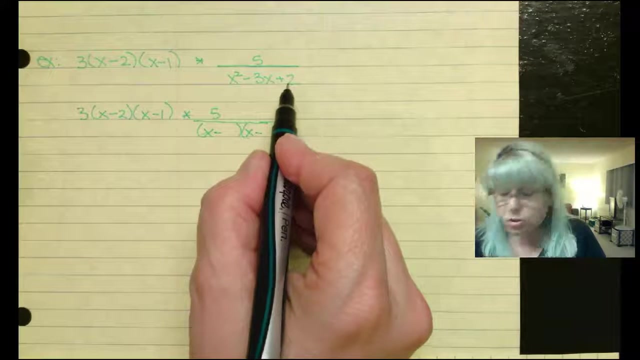 If possible. Okay, Three X minus two X minus one Times Five All over. I know they're both The same Sign And both of the signs are negative. Uh, One and two will Multiply to two.